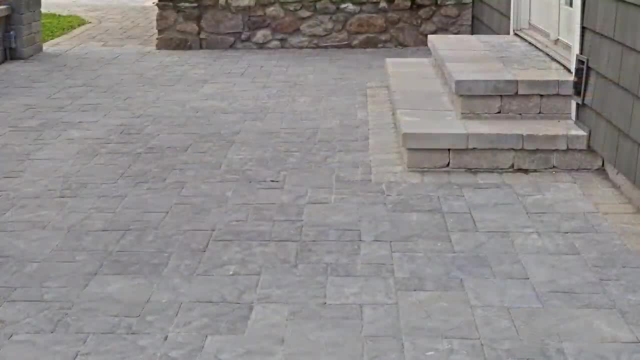 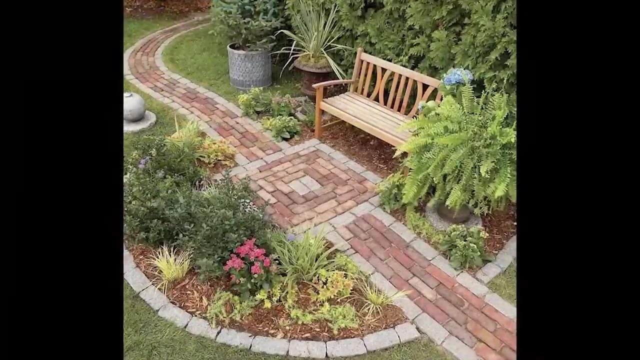 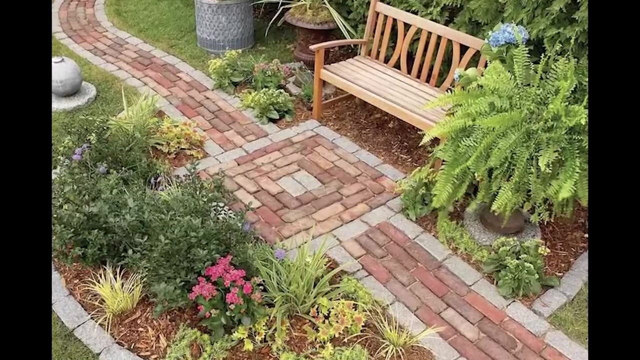 area or design. Most of the time, people use them in high traffic areas like patios and driveways because of their durability. But pavers don't always have to have a practical function. They can be used just for their visual appeal. They will make any garden or pathway look more attractive. 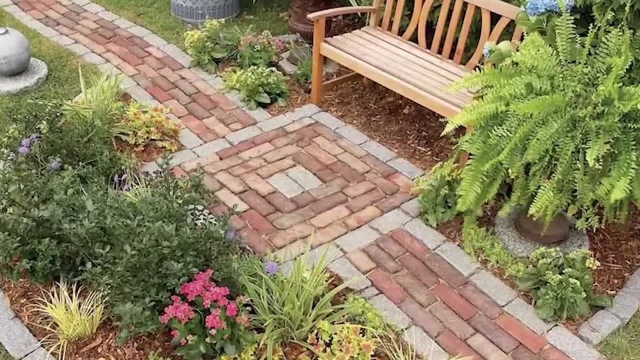 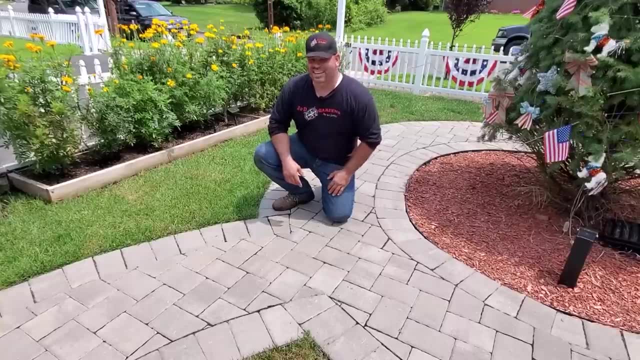 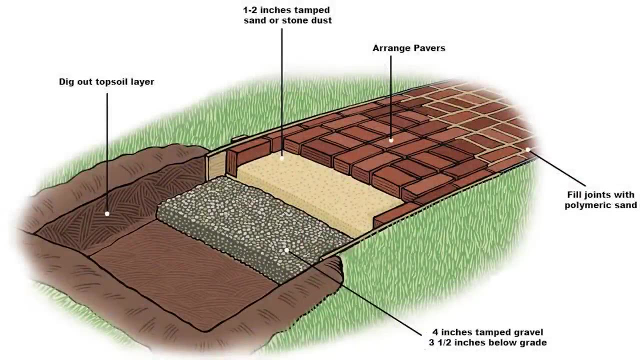 cleaner and tidier than grass or dirt ever would Now. pavers are a great option for walkways, but for those who aren't familiar with them, it can be a pretty big process getting them installed. In order to install pavers correctly, about eight inches of topsoil will need to be removed to. 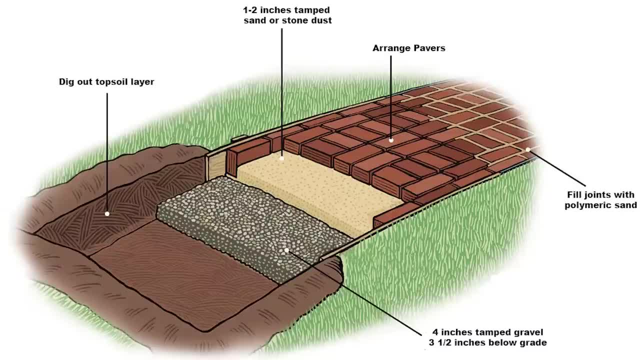 create a base or a foundation for your walkway, Three and a half to four inches of tamped gravel will need to be added, and about two inches of stone dust for a smooth surface. From there, pavers are arranged in a desired pattern and then secured with edging, and 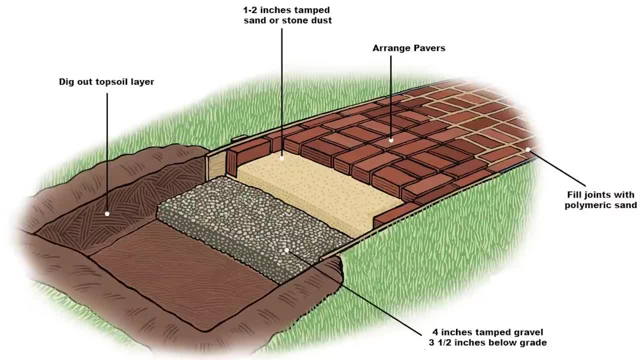 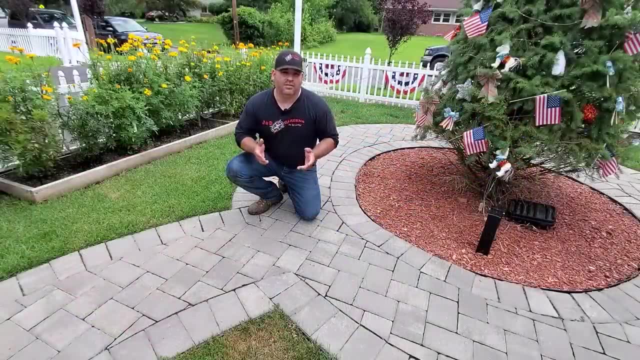 polymeric sand for the joints. Digging the pavers into the ground will allow for the walkway to be level with the surrounding garden. So, as you can see, it's quite an involved process and, depending on the size of your project, it can get kind of costly. 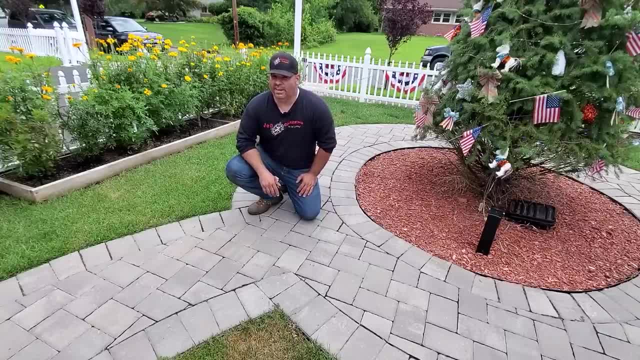 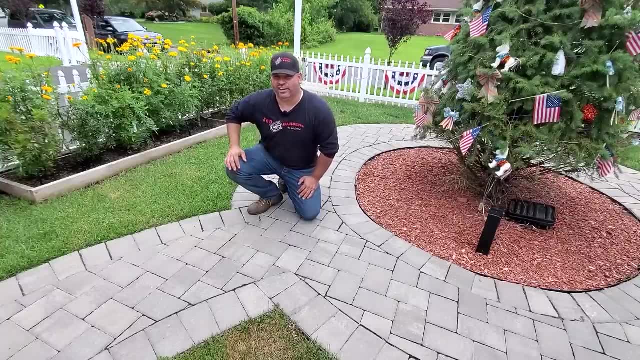 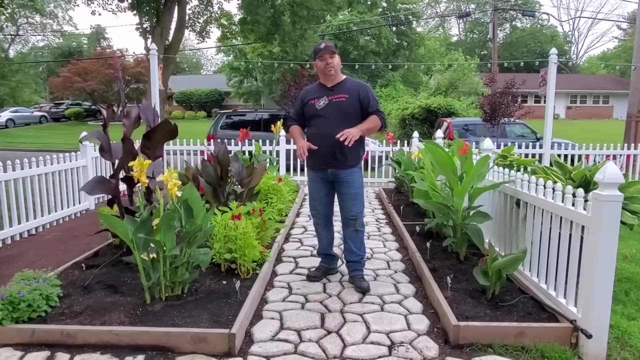 But if that's really not in your budget, I do have a way of making a great pathway. that's a total DIY project and it won't break the bank. Let's head over to Garden East. Okay, so we're here in Garden East and, as you can see, we use the more traditional style walkway. 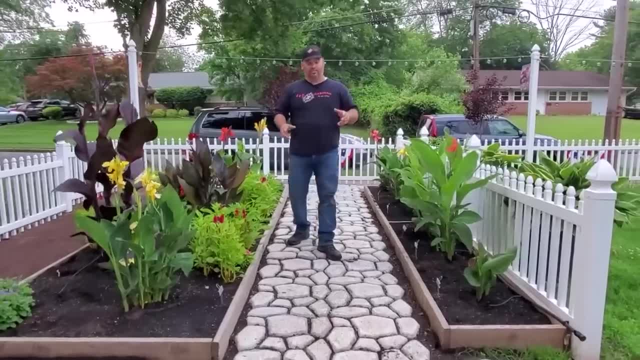 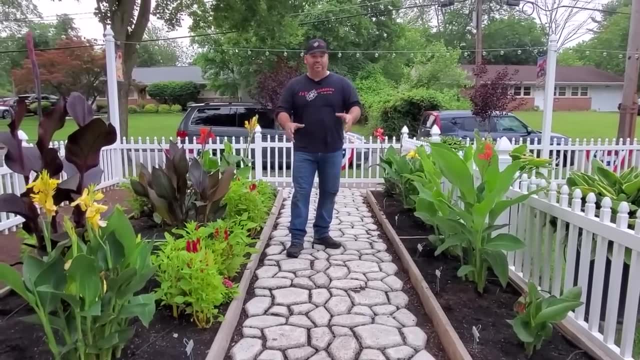 around our planter beds. Now, at first glance you might think, wow, Dan, you got a individual stones here. You got nine different styles. This is crazy. This would be like a giant jigsaw puzzle to do, But actually it's poured concrete using a template. 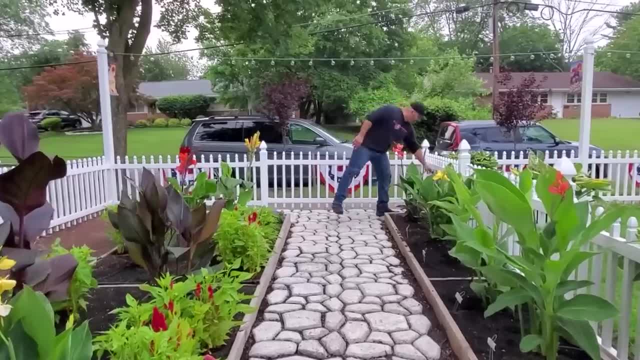 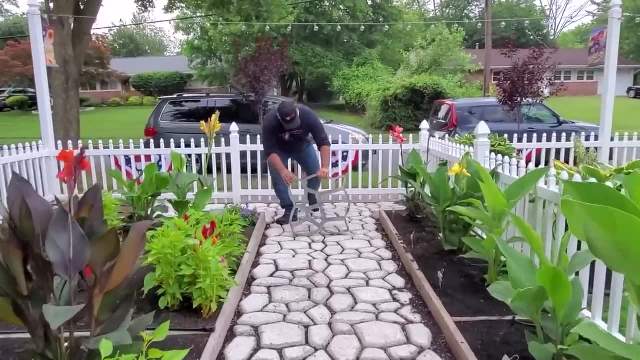 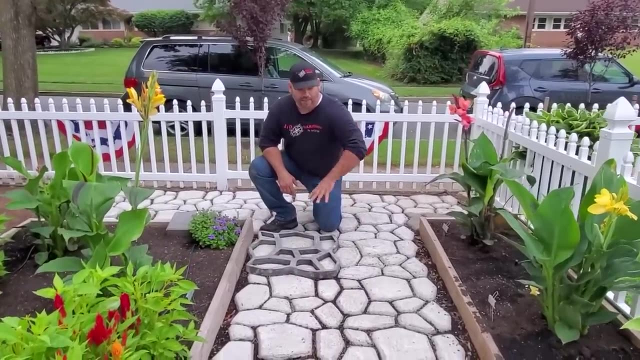 system. Let me show you. This is called the Quikrete Walkmaker and what it is is a template that you pour concrete into. Let me line it up for you so you can see. the template matches the style. Now this style is actually called. 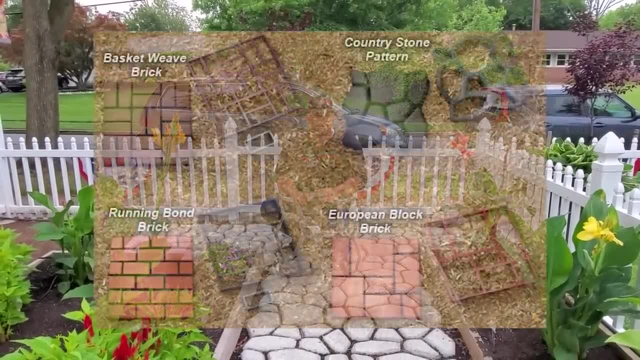 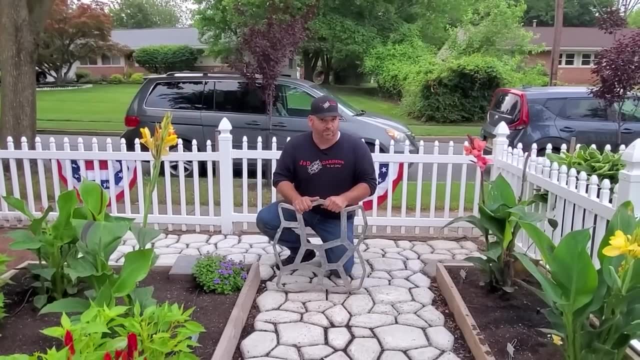 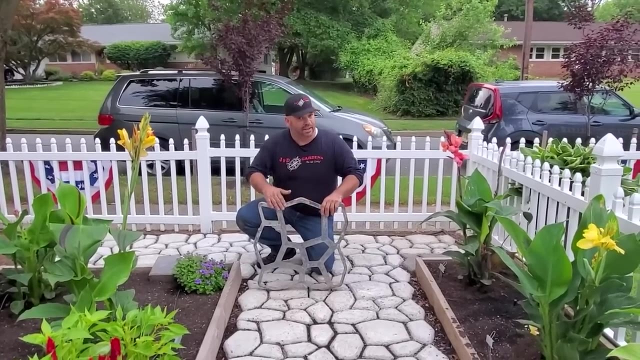 Country Stone, but there's a few different styles, So you can see, you can choose a style that's more to your liking if you don't like the more traditional look. Now, it's a very simple system. I'm going to have Jackie demonstrate it in a minute, But just to warn you, there is some. 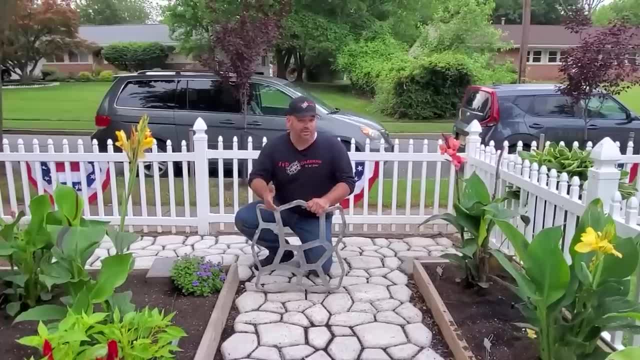 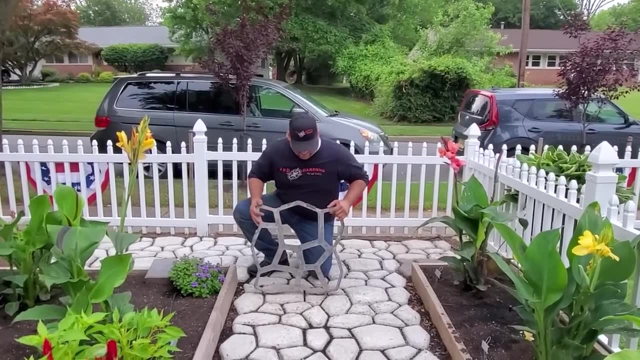 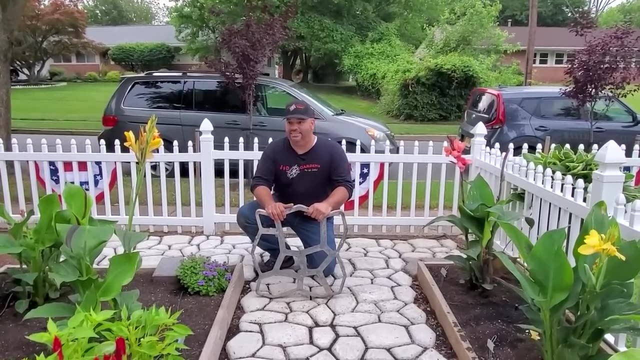 labor involved. There's- uh, it can be a little time consuming, depending on how much path you're doing, and some a little bit of backbreaking work. I mean, each template you use an 80 pound bag of concrete. So if you think about it, today we're going to be doing around 32 bags, and so that's. 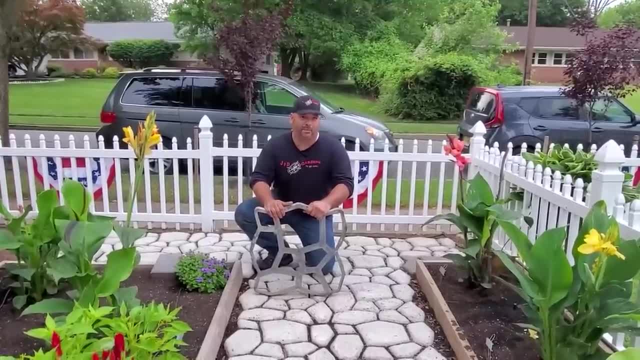 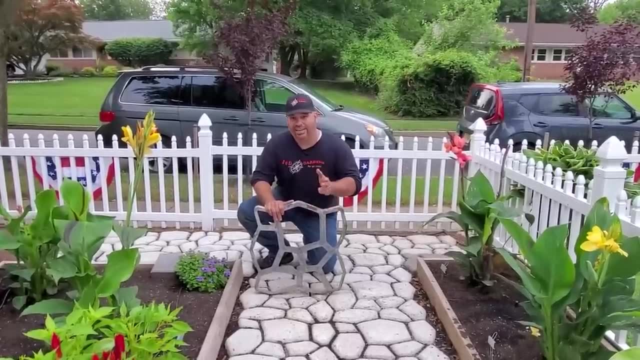 going to be about a little over 2700 pounds that I'm going to be lifting and moving around, So there is some work to it, but the results are great. So, uh, and you can save yourself a ton of money. Give me an example, like the pavers that I showed you before in Garden West. 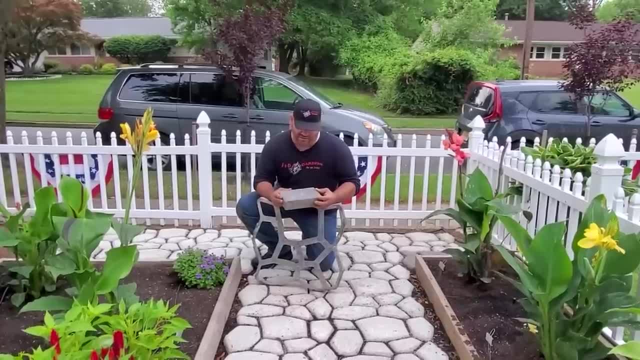 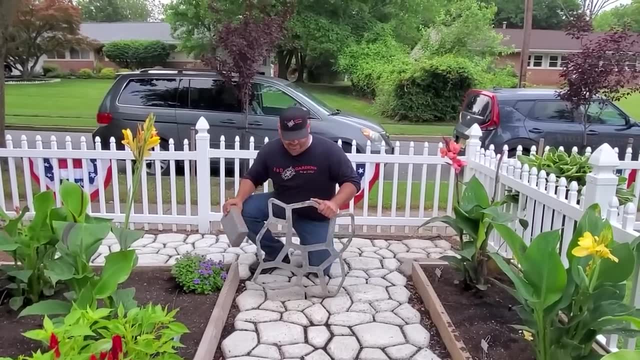 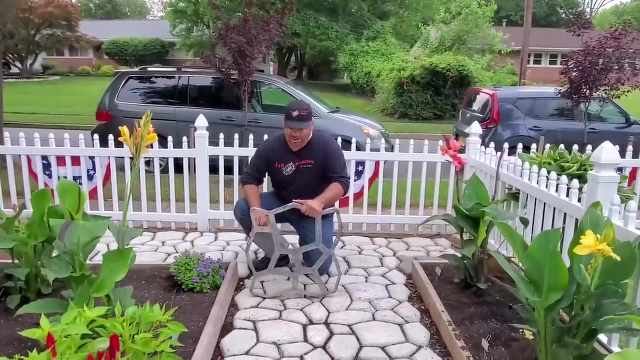 Each one of these, uh, it's about nine by uh, uh, six by nine uh. each of them about a dollar, And you would need about uh eight of these to fill up this template, And an 80 pound bag of concrete costs around uh a little under four dollars. you could probably get it for So. 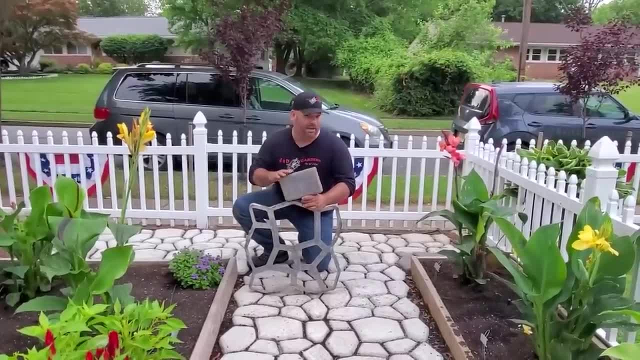 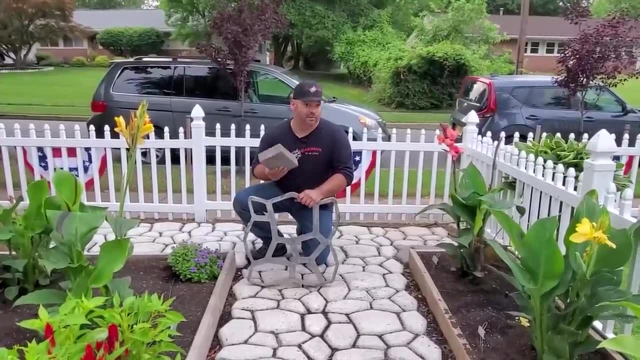 you can see the savings and that's just, uh, this, just about a dollar, just for the stone, Not including the crushed, uh, crushed gravel, uh, the stone, dust and obviously the labor to do it. if you don't know how to do it, This is truly a DIY project. So, uh, we'll show you in a second. 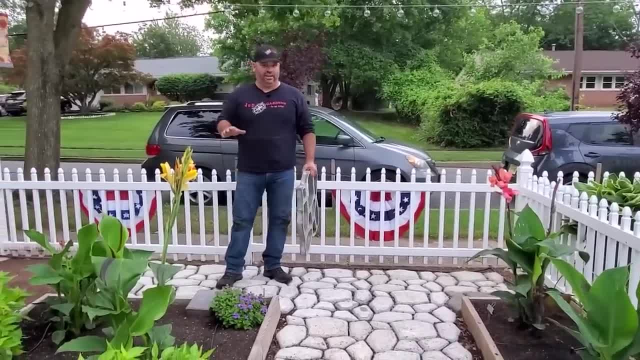 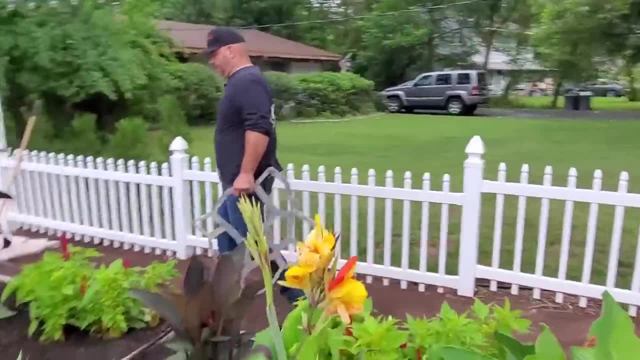 So In the beginning of spring we actually redid Garden East, So there still is a a fair amount that we have to do. If you want to bring the camera around, We have this whole back section that we're going to be doing today. 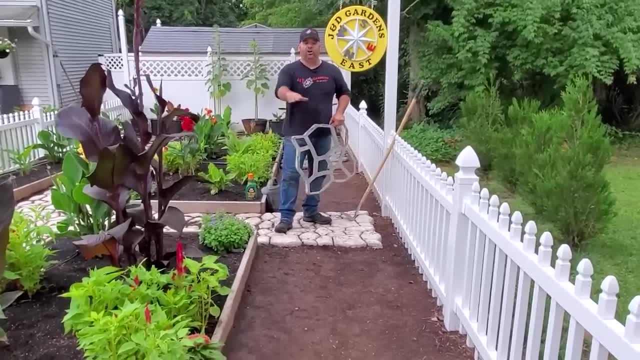 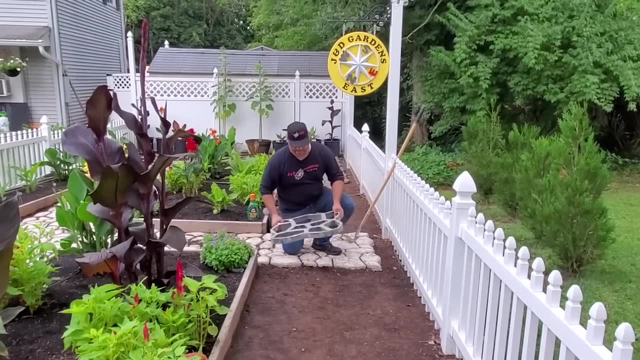 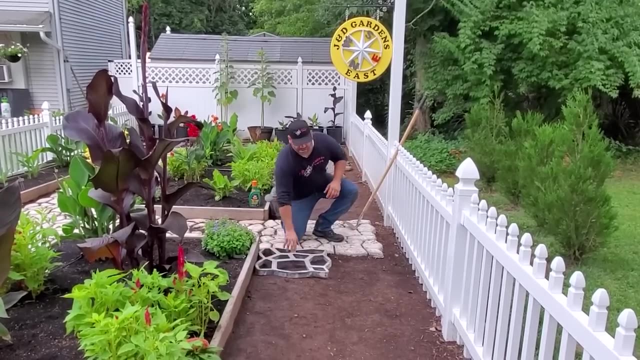 So, before we get into that, let me uh talk a little about the prep work that you have to do. Now. the beauty about this system, it's it's what's called like a self-leveling system, Meaning once you place- let me get the right way out here- Once you place it on the ground, because it's a sturdy, it's a sturdy. 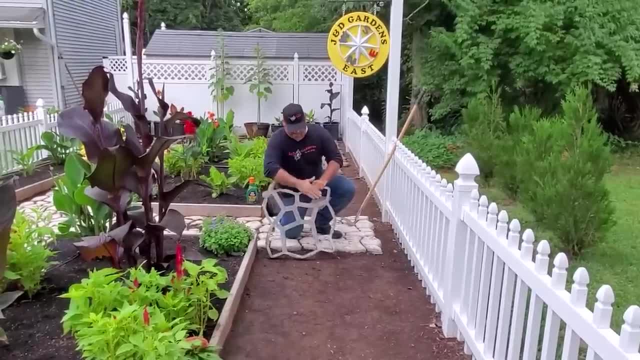 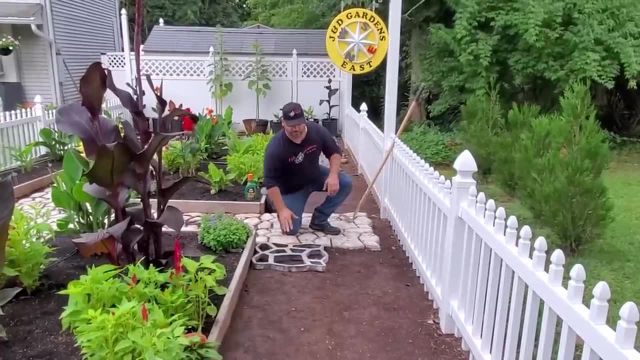 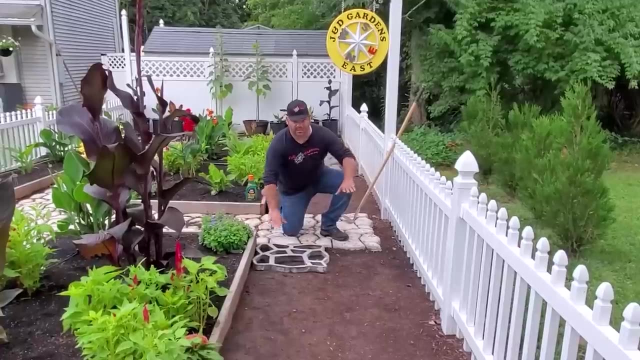 uh, plastic form, it stays perfectly level on the top. So, even though your ground might not be perfectly level, the top will always stay level And as you pour the concrete, it will fill in all the little gaps. So it'll be nice and smooth and flat on the top. But, like I said, there is some. 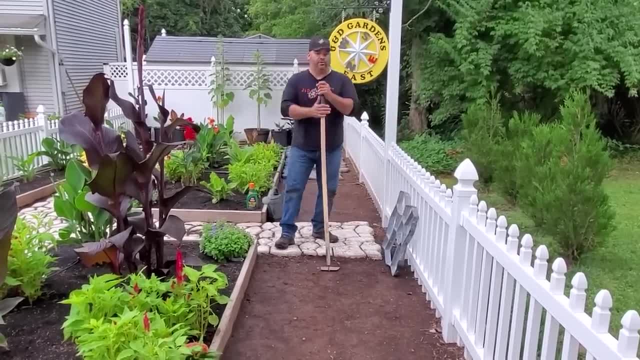 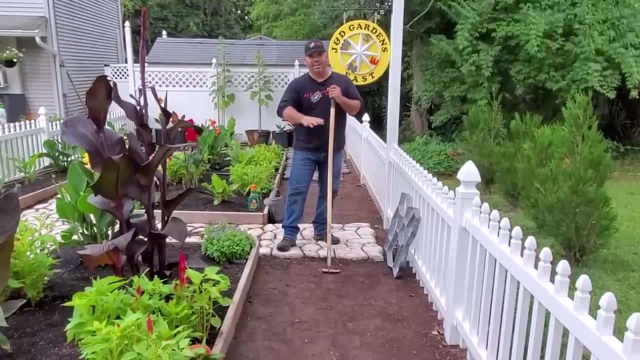 prep work you want to do First, depending where you're doing it. If you're doing it on grass, you want to obviously pull up the grass that you're doing. If you're doing it anywhere else, you just want to try to get it as. 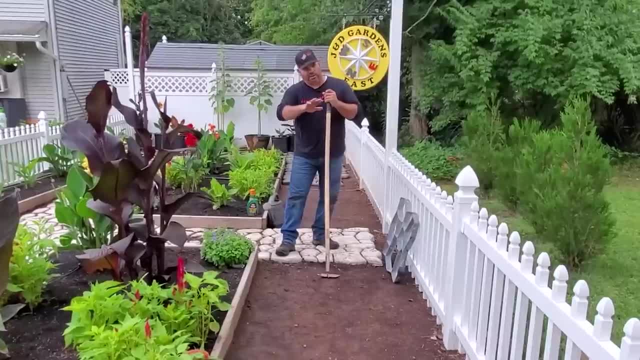 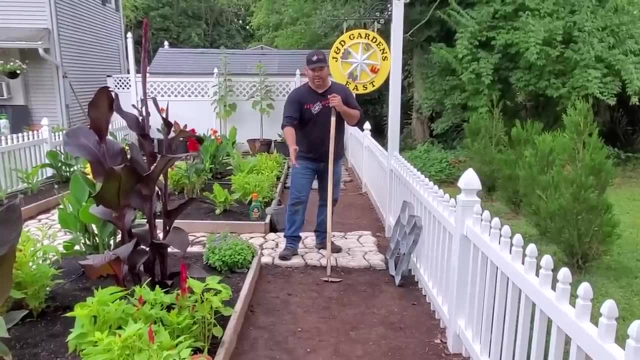 smooth as possible. It doesn't have to be perfect, But you want to put a little time into it. The more you put into it, the better it's going to come out. You want to get rid of any kind of weeds or any kind of growth that you have, And what I like to do is I like to use a hoe And 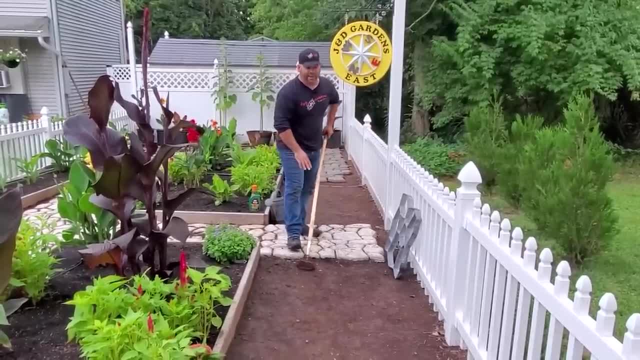 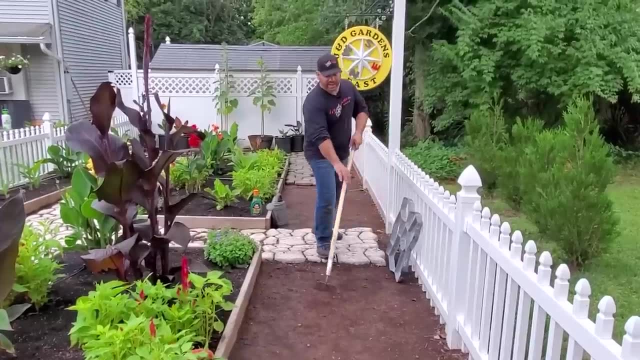 I just scrape it down. I've already done this, so I'm going to show you. I just like to scrape it down to get it in the ground And get it as flat as possible. If you have low spots, you move all the dirt over there And you just get in. 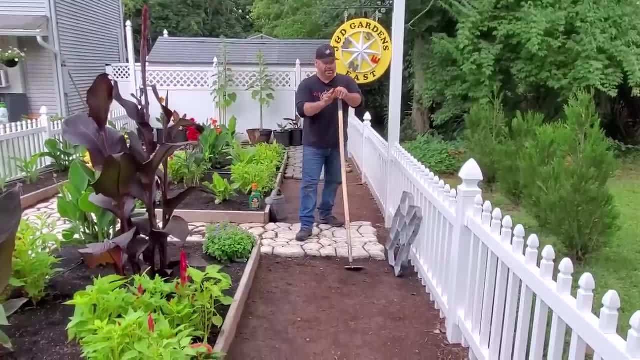 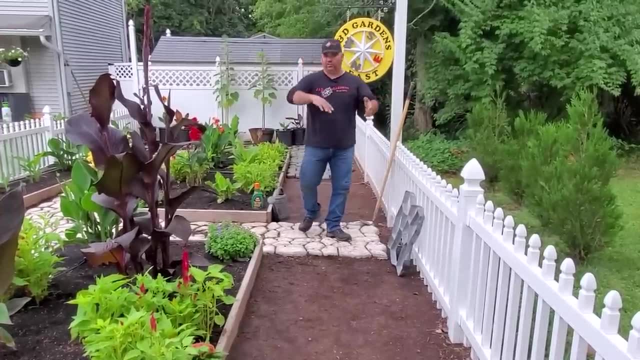 You look at it with your eye and say, yeah, okay, you know, that's pretty level And that's good. The template will take care of the rest. Now the other thing that I like to do before I get started. I usually do this the day before, But we have two sections, so I already did that section, So I'll 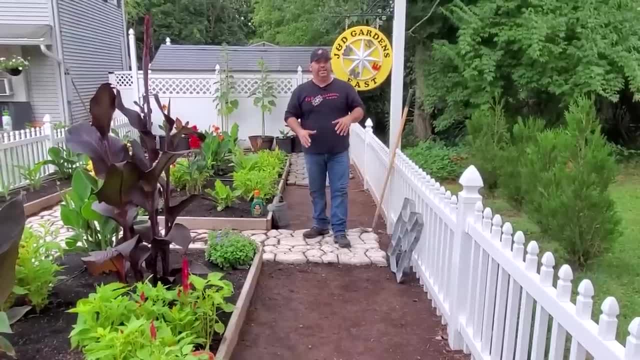 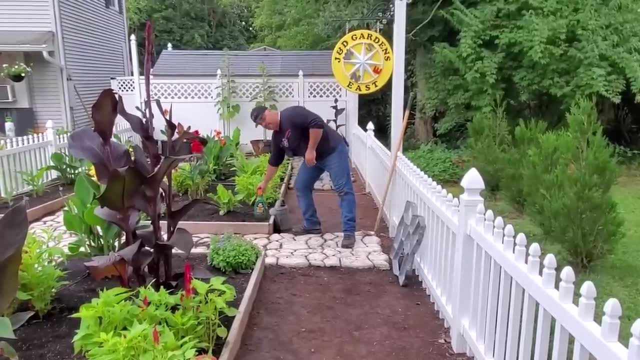 do this section Is. I like to use some kind of ground clear in the area. I want to make sure that any kind of growth is killed underneath it. I like to use- and there's different ones, But this is what works well for me. It's actually ortho weed. 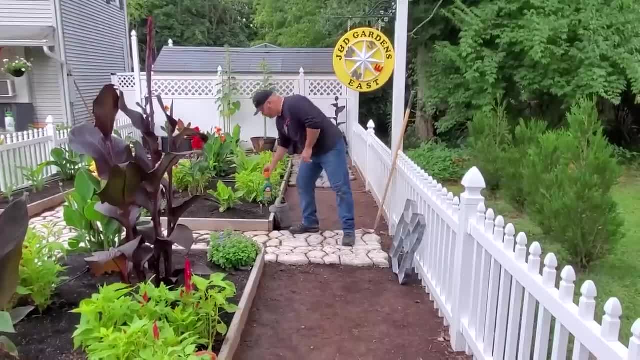 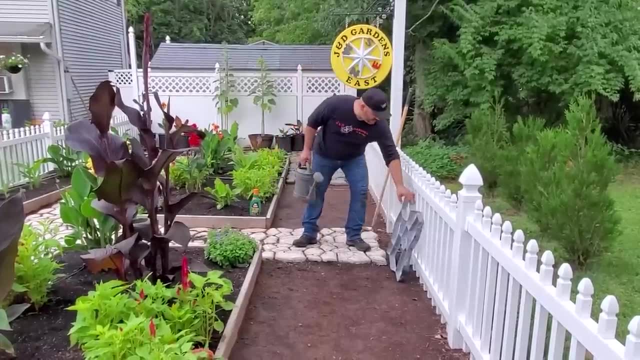 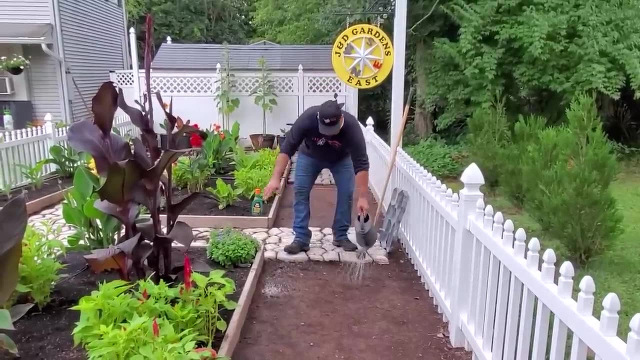 weed, clear lawn and weed killer. And you can use a spray bottle. I actually like to use a watering can Because I like to be give it, be very generous with it, Because I really don't want anything growing in between. So what I do is I pour get close to plants And I really lay it in thick. 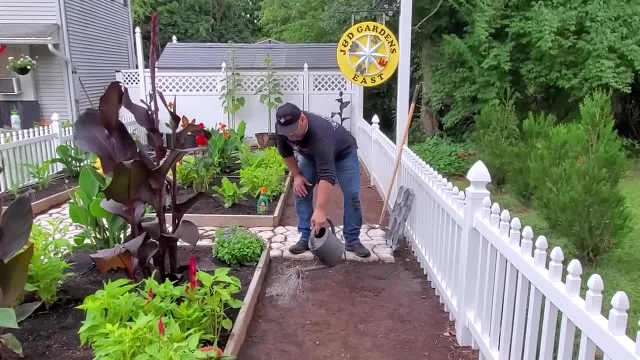 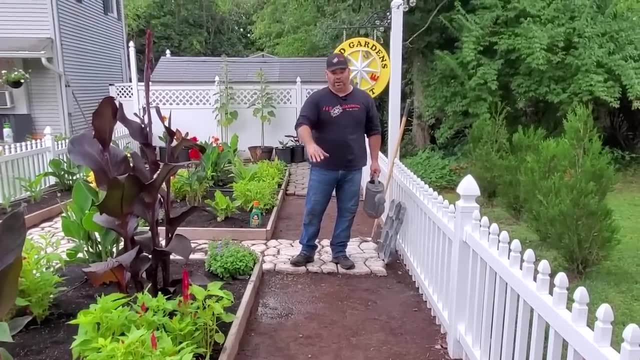 And if you have to use a little more, that's okay. So there you go, All right, and now. what I'm going to do now is I'm going to cover the whole area, Probably have to make another batch of this, And then what we'll do is we'll set up everything that. 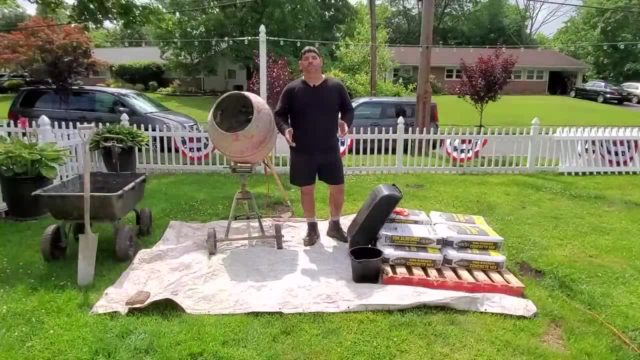 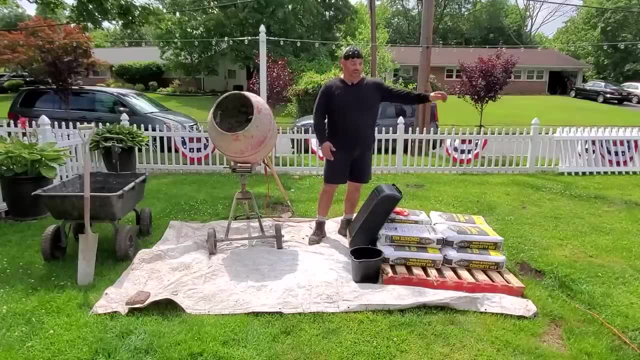 we're going to need to start the pathway. Okay, so we're about ready to start mixing our concrete for our pathway. A few things: We got our bags of concrete here ready to go, We got more in the driveway, We got some fresh, clean water And we've also added a tarp to protect the grass. 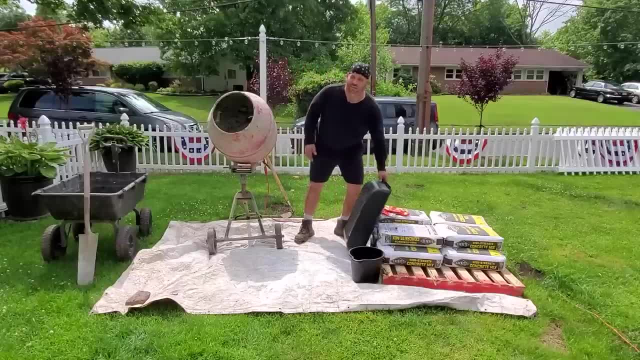 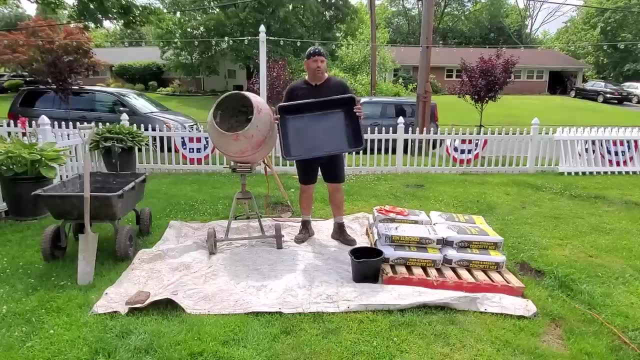 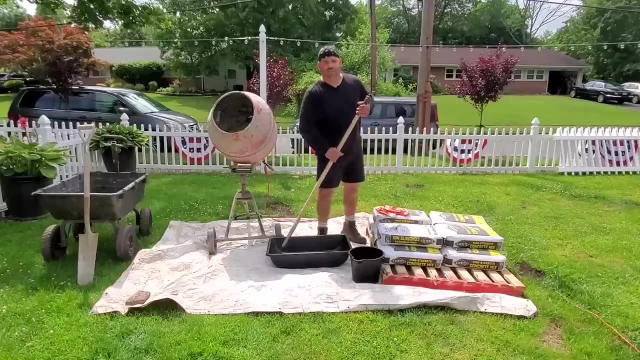 village. Now one way to mix your concrete is to get a trough like this. You can get these at Home Depot or Lowe's And it can hold an 80 pound bag of concrete. And it's pretty straightforward: You add the bag of concrete, Add the water And use a hoe And you can mix it up. Get the 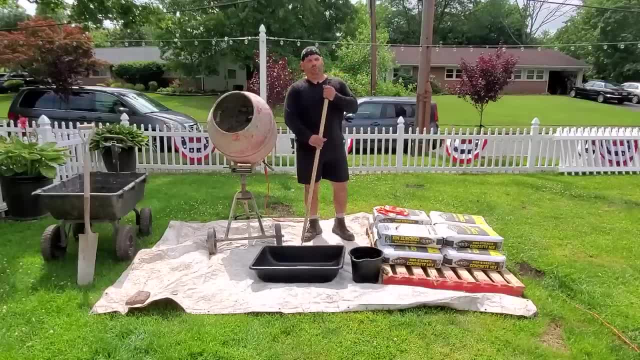 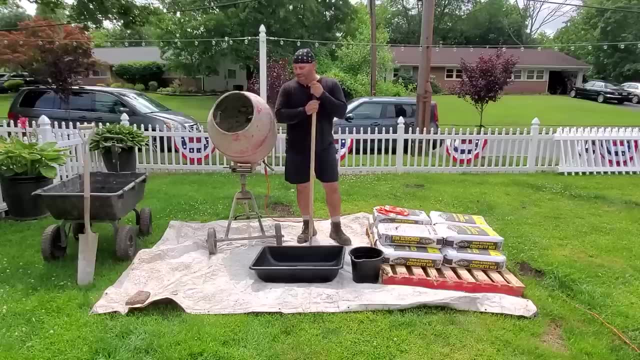 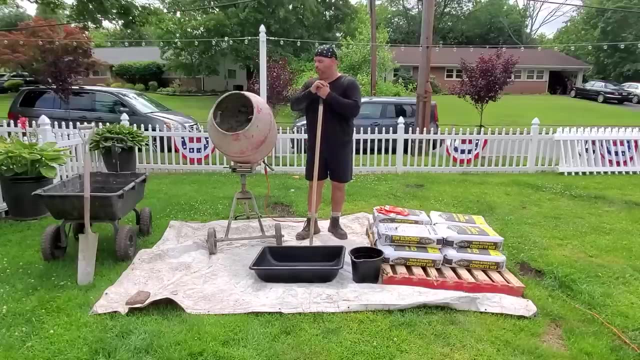 consistency that you need, And that's fine if you're doing a small amount, But if you're doing a large amount, like we are today, You might want to consider getting a cement mixer. Now rent these, I think, it's every for four hours or for the day, And it's a lifesaver If you're doing. 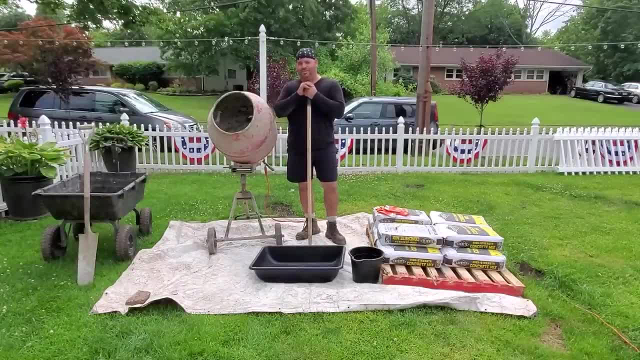 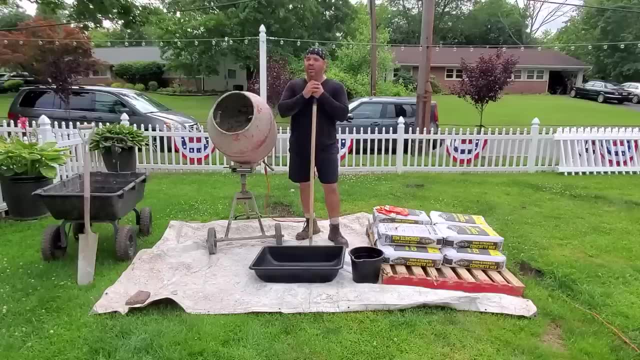 a ton of bags. You really might want to consider that. One other thing you might want to consider is, depending on how much you're doing And how much time you have, And, if you're, whether you're doing it alone, You might want to consider buying one. Now, I know that sounds a little silly. What? 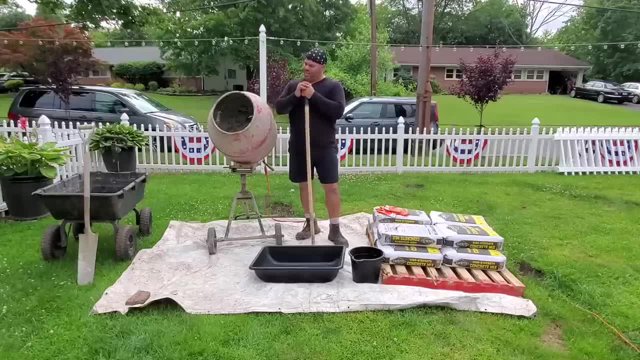 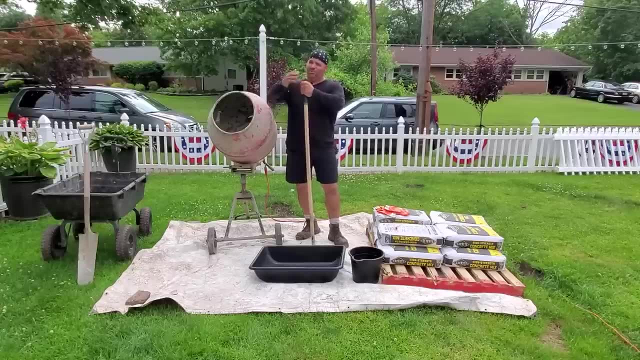 am I going to do with the cement mixer? But think about it. To rent the cement mixer like this, It costs close to a hundred dollars for the day. Okay, so if you were doing like 30, 40 bags or more, You know it could run into the second day. So you're going to be close to two hundred dollars. 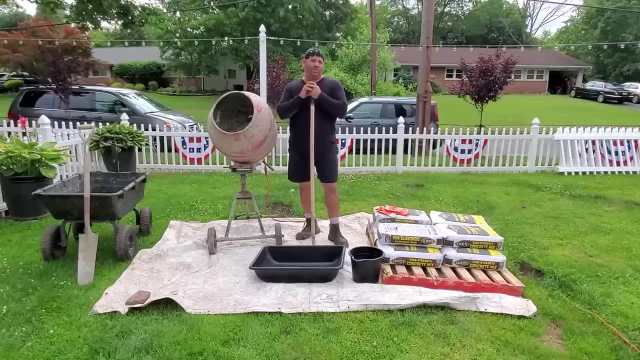 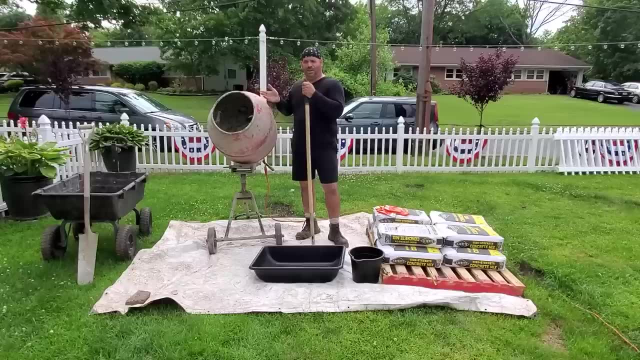 A cement mixer like this costs about three hundred dollars, And they actually make smaller ones. So if you do the math, You might want to consider that, Because the if you- uh, if you have it, Then you're not under the gun That you got to get it back to. 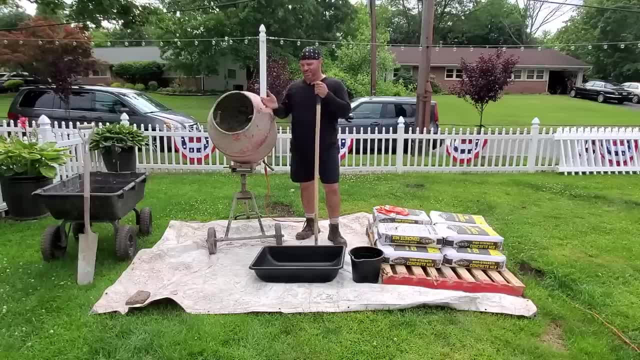 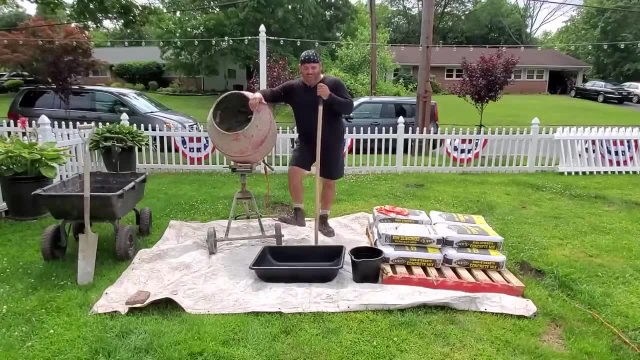 home depot via charge for the extra day. You can work at your own pace And if you don't finish it, you can do a couple of bags every day. That's the beauty of owning it, And if you have a lot of other concrete work you're going to be doing in the future, Uh, it's uh, really uh, something You know. 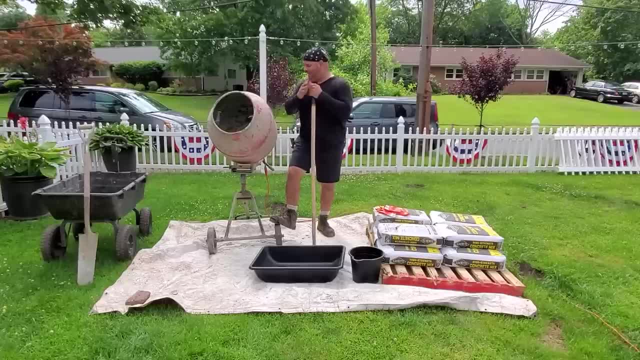 obviously, if you have the space And if you want to spend the money on it. I mean, I've had this uh concrete mixer for about, uh, I think, close to 15 years And it's great. It's electric, So I don't. 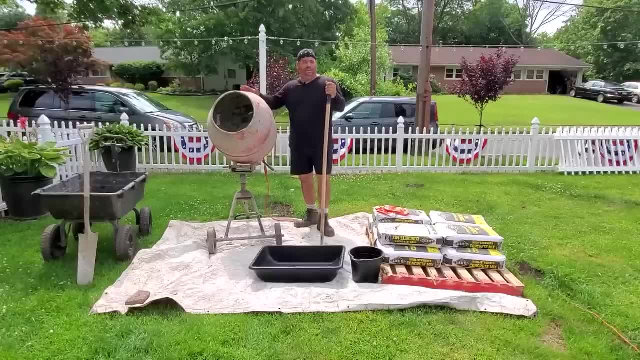 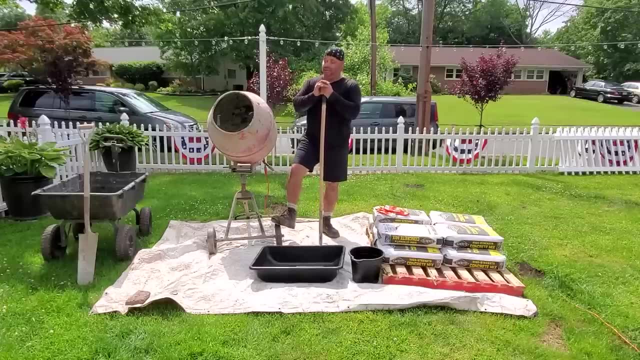 have to worry about anything. It's not gas powered And uh, it's been a trooper for me. So, uh, just something to think about. Just kind of weigh out how much concrete work you might be doing in the future And whether you have the space to store it And, at the end of the day, if you have a large 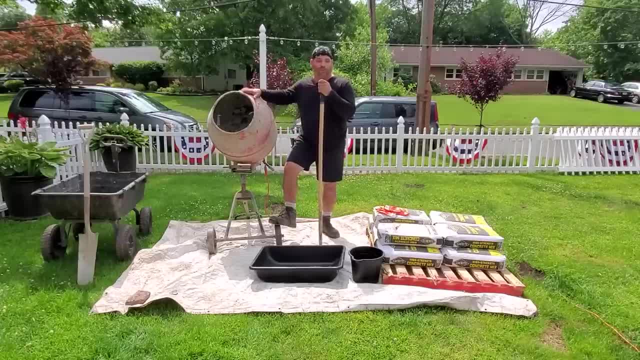 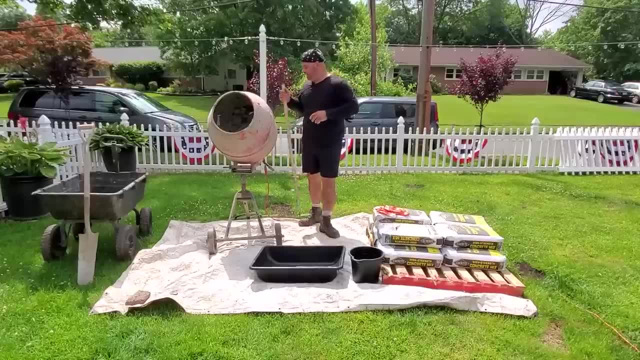 project. Uh, it was still probably cheaper to buy it. And then you can always try to sell it, uh, down the road If you don't have the room for it. So just think about it Now. another thing is- I'm going to speak from personal experience here- Is: uh, if you're not used to working with concrete mix, 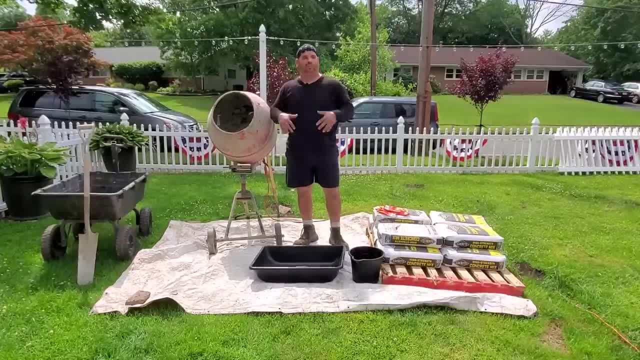 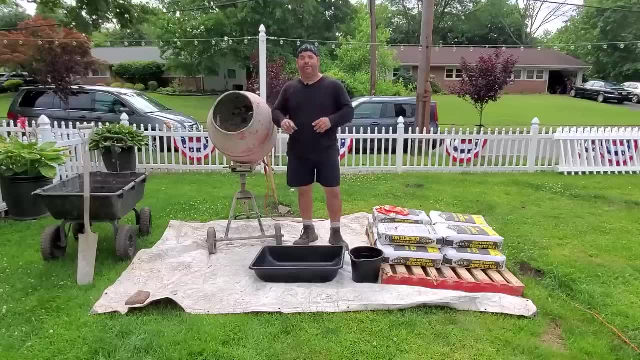 Uh, concrete mix, You might want to. you want to make sure that you're protected. Now, of course we've. uh. one other word of advice: Don't pick the hottest day of the year to do this. You want to do it on a cooler day and start early, Because I think it's 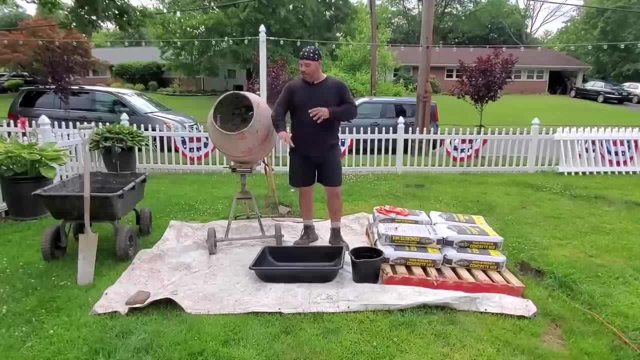 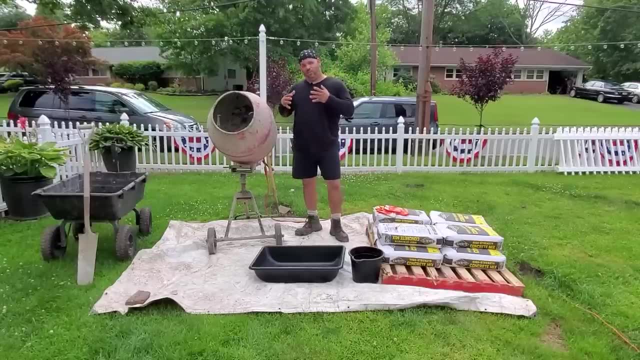 going to be hitting into the upper 90s And it's going to be terrible, But it's important that I'm covered- Long sleeves and uh and a long heavy shirt Because, uh, with working with concrete, There is something as concrete burn or chemical burn, And it's actually happened to me, I think. I 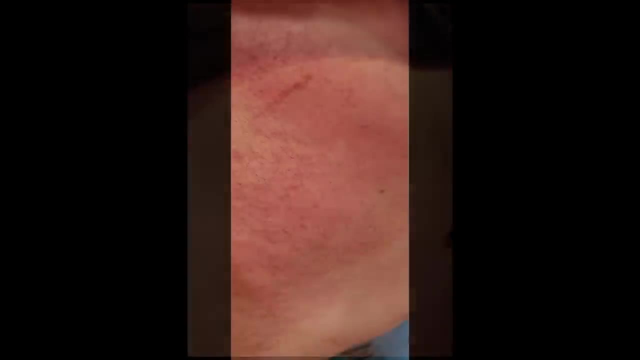 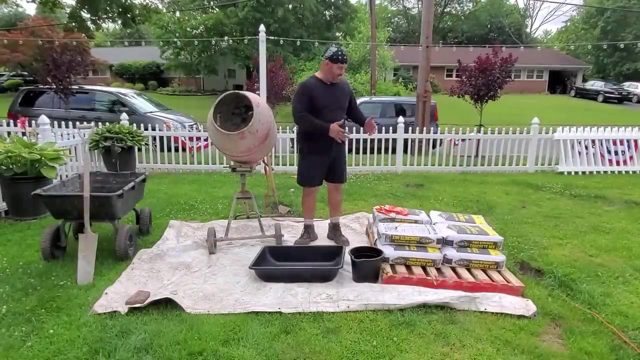 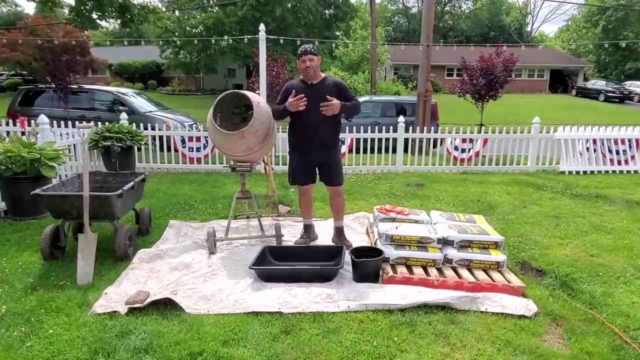 have a picture of it. So when you're working all day And you're mixing about 32 bags And you're going to be sweating And the water and everything's going to be getting where, It's very easy to get burns on your arms. 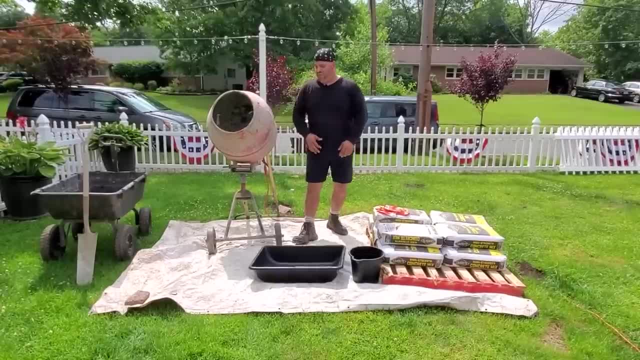 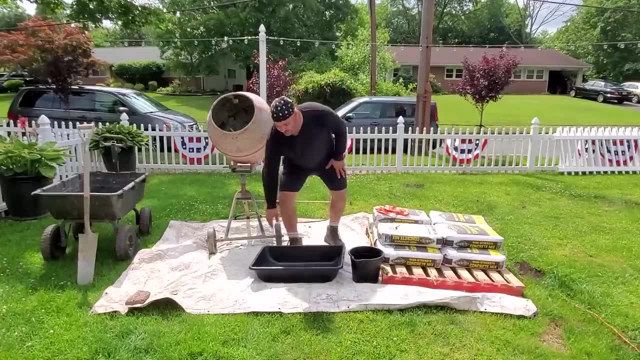 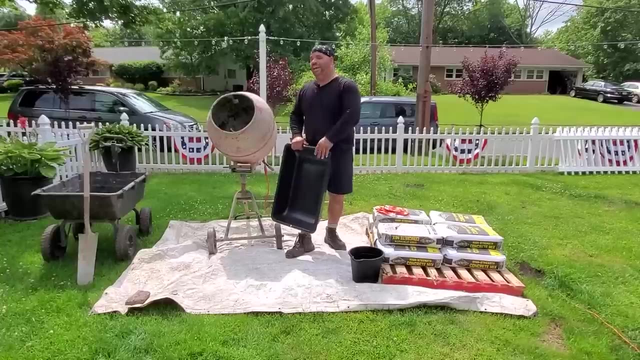 And on your, on your torso, It and it's happened. So, with that being said, Let's uh get started. Make sure it's working, okay, Perfect, all right. So, uh, Jackie's over here in, uh, in Garden East. She's going to be doing the forms. I'm going to mix it out here And I'm going to 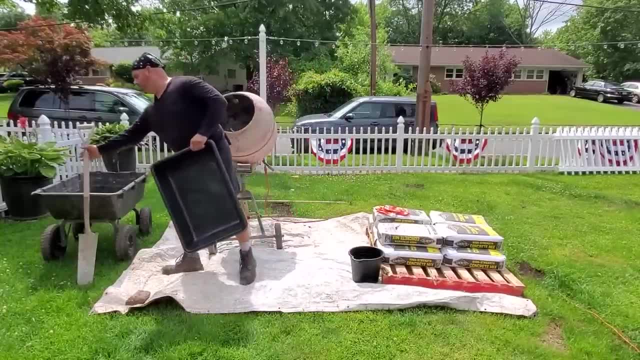 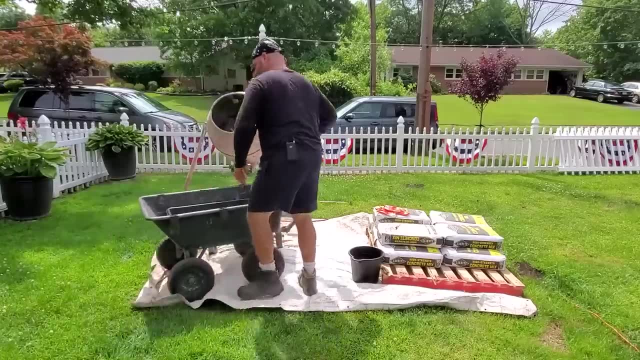 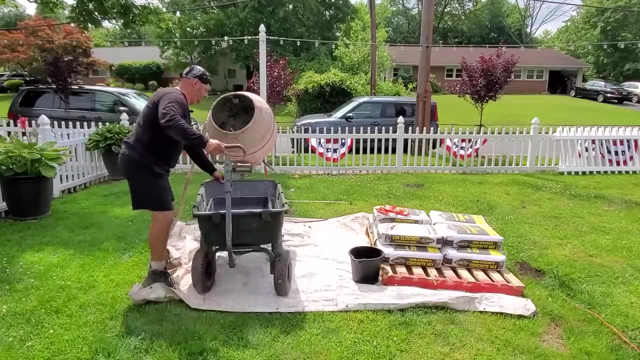 transport it over to her. So what I'm going to do Is I'm going to take my cart here, I'm going to add Whoop, excuse me, I'm going to add the little trough inside So I can pour it right into there. This actually pours right down. 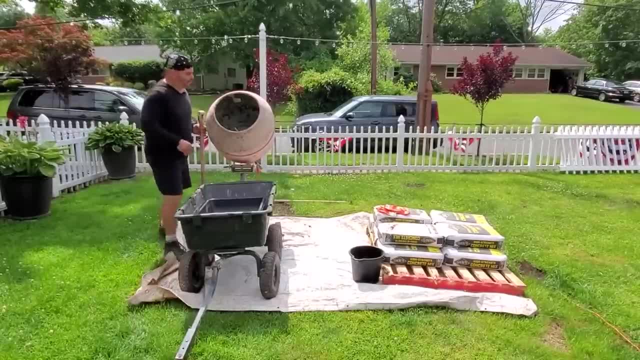 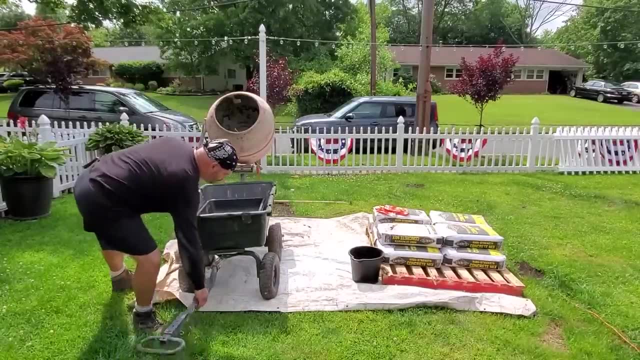 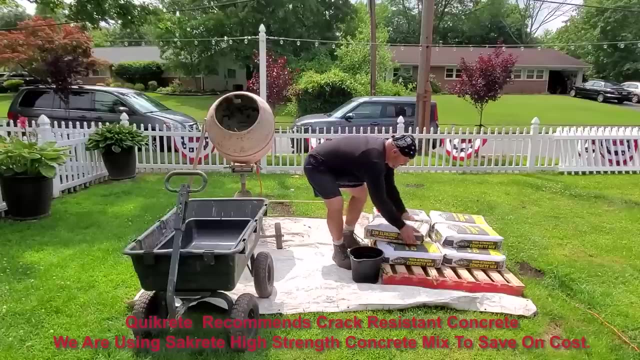 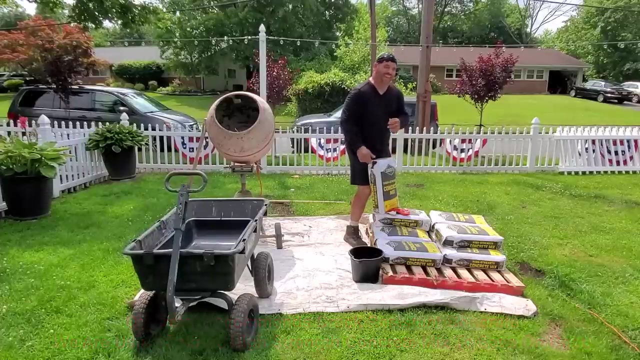 And then I can transfer it. I'll wheel it right over to her, So I have a little scoop in there. So before we do that, Let's- uh, Let's- get the bag of concrete. This is the fun part. So always have a razor with you, Don't just rip it off from the top, Because 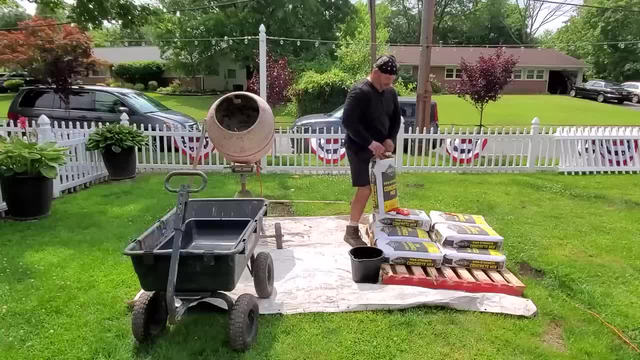 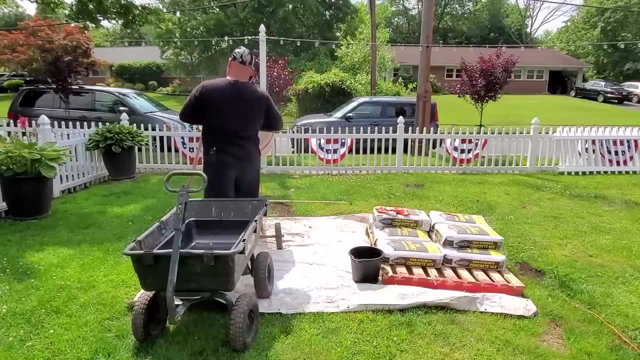 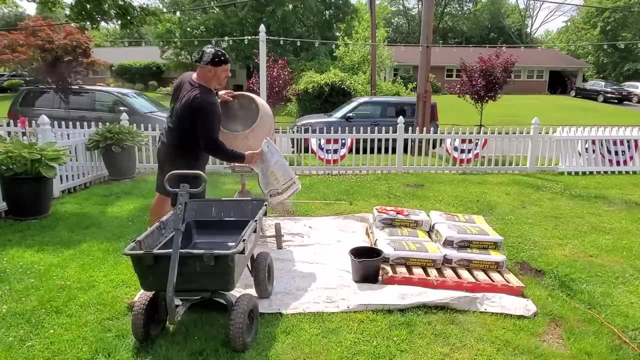 then it's going to go over. You want to control as much as possible, So, okay, Now I'm going to do one bag at a time, Because I'm going to be transferring it over to Jackie, So hopefully you can hear me as. 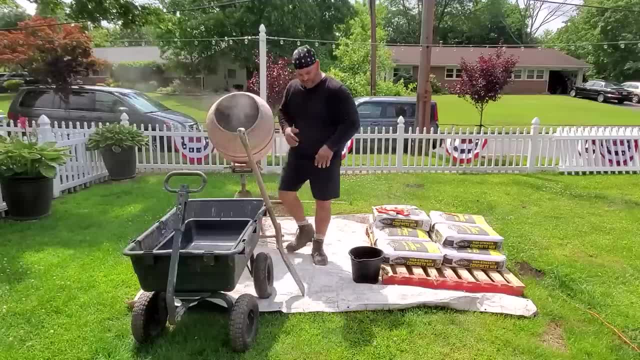 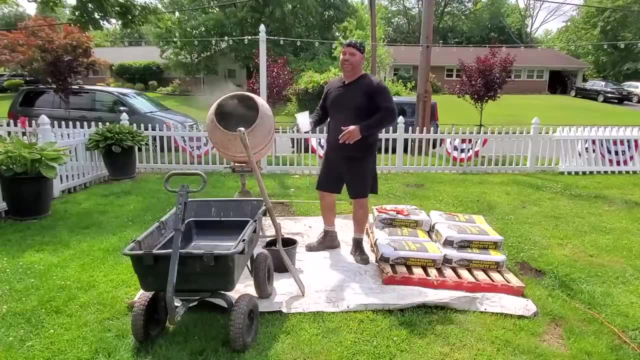 the cement mix is going Now. if you read the instructions It says three and a half quarts. Normally I will just take a water hose And I've been doing it for so long And I just kind of know how much do it. But I'm going to do it correct way for you all. 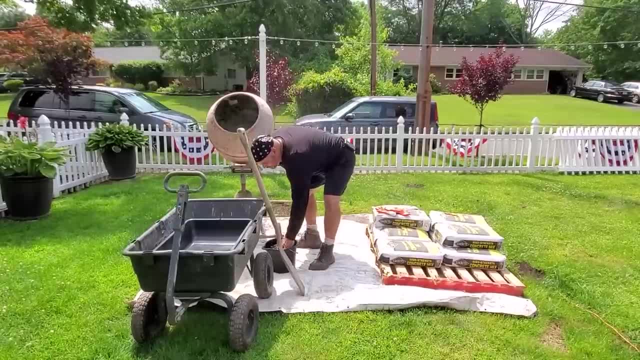 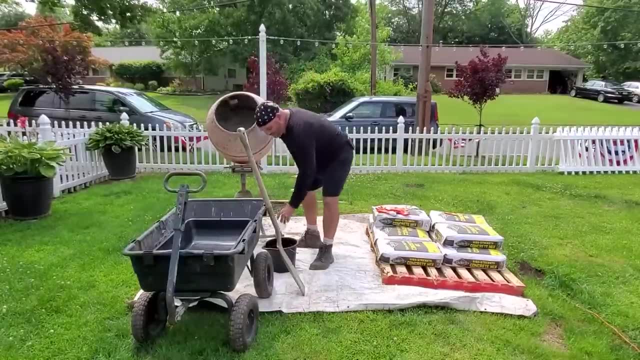 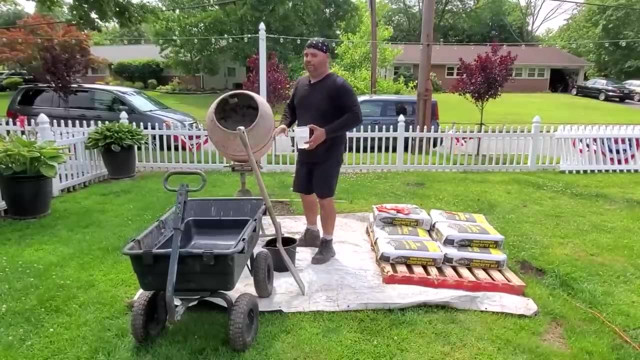 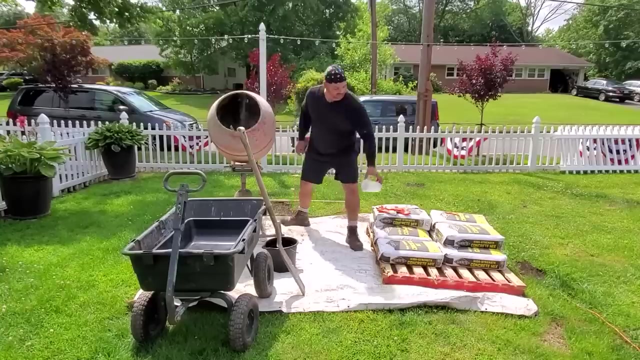 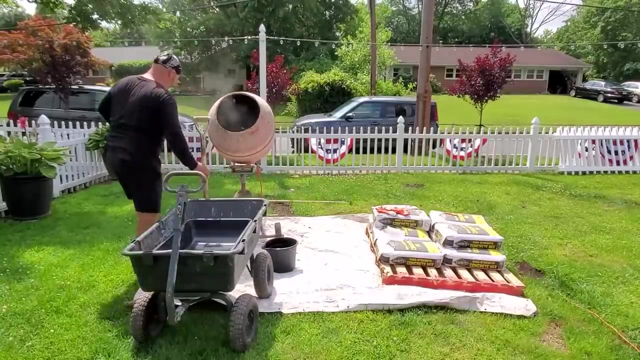 I have a quart here. I'm going to fill it up here. Three and a half. I find that usually need more, But I'm going to do what it says for now. We'll start mixing and I'll make sure it gets mixed up. well, it's a lightsaber, trust me. okay, so just. 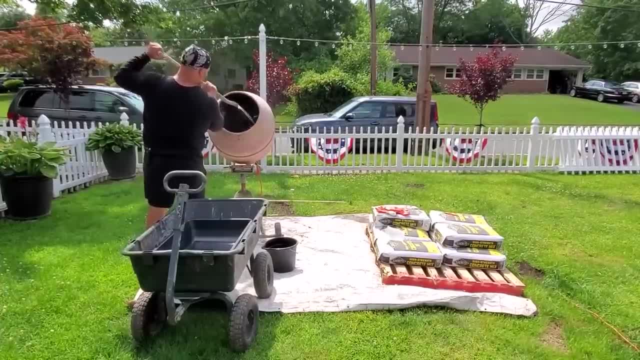 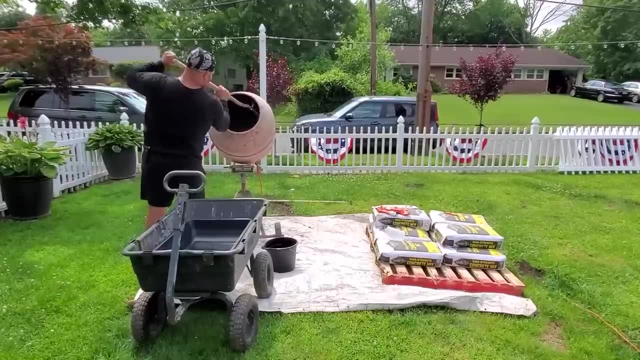 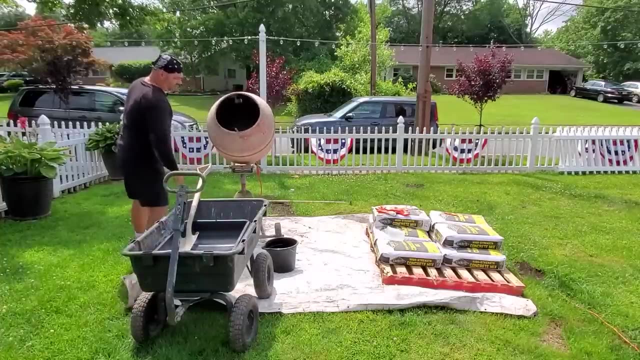 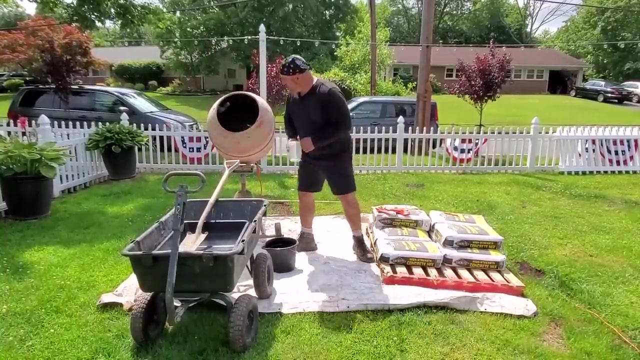 want to make sure now we actually want it to be a little more look, we want it to be a little more soupy because it's easier to work in the form. so I can see that three and a half quarts it's not going to cut it. 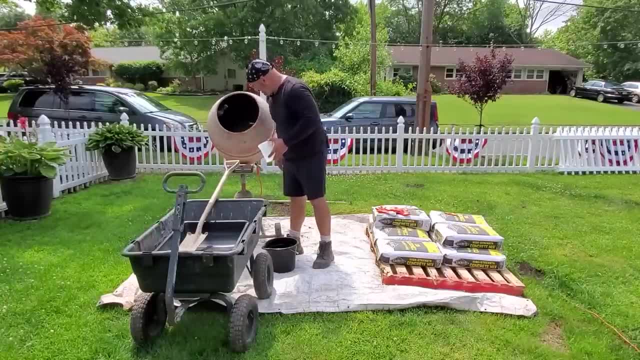 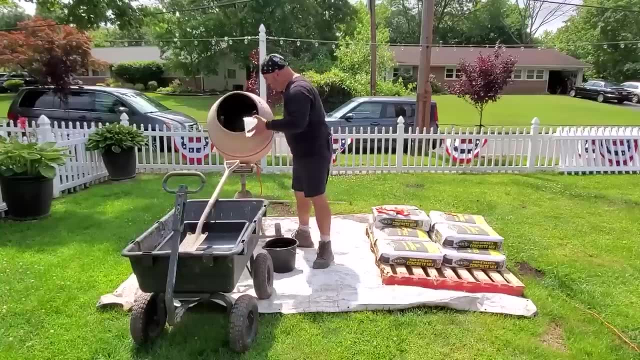 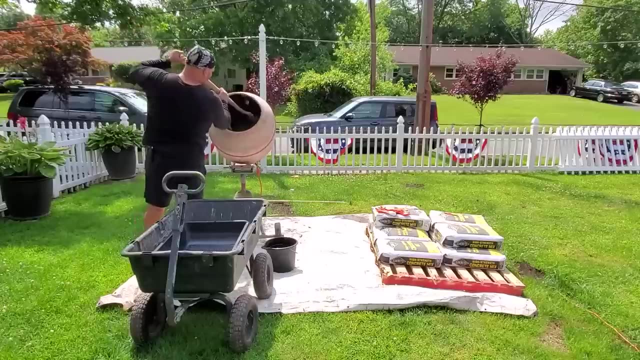 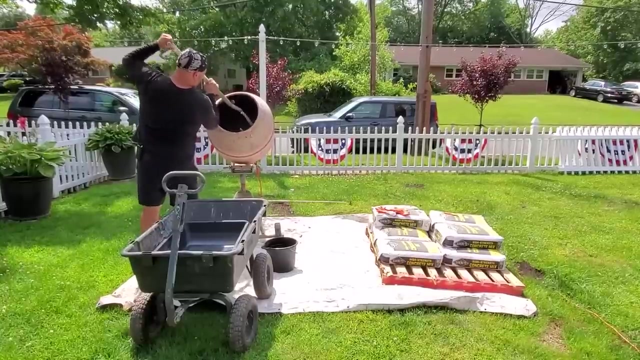 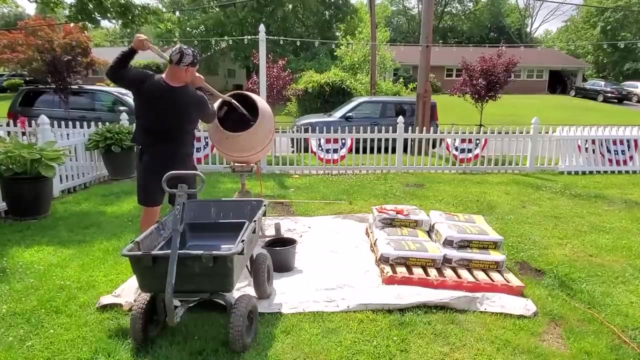 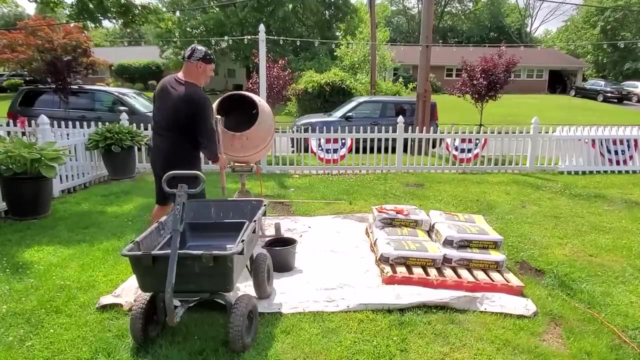 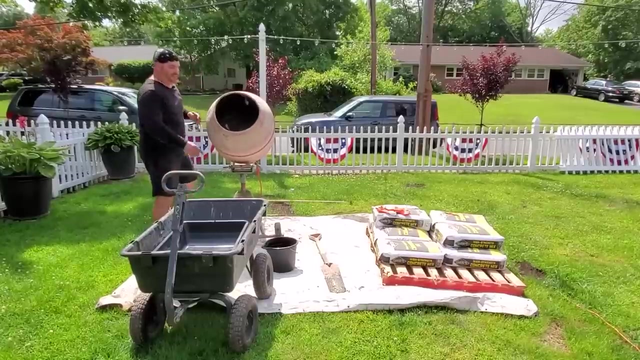 it's getting there right now: four and a half, and this will probably do it five and a half. you don't want it too soupy because you have to work it, but it's getting there. I don't think we're good now. the reason I was using a shovel, because if you've ever worked with a cement mixer, 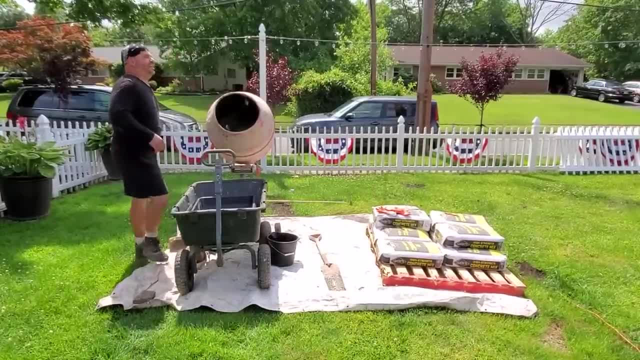 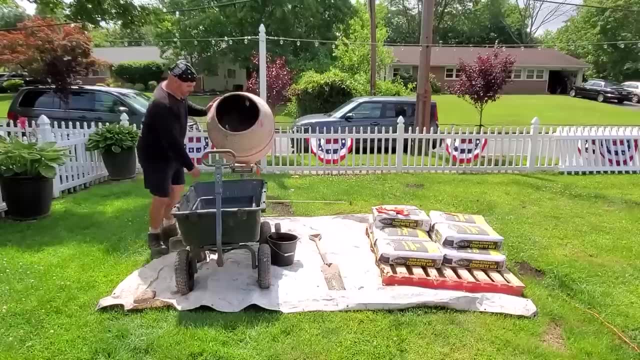 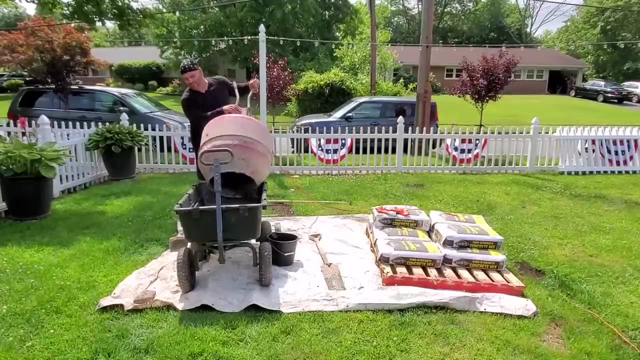 it's very much like eating peanut butter sticks to the roof of your tongue, and it does the same thing inside a cement mixer. so, okay, okay. so now I'll dump it right there, and I usually turn it on to make sure it dumps everywhere- everything that's inside, rather. 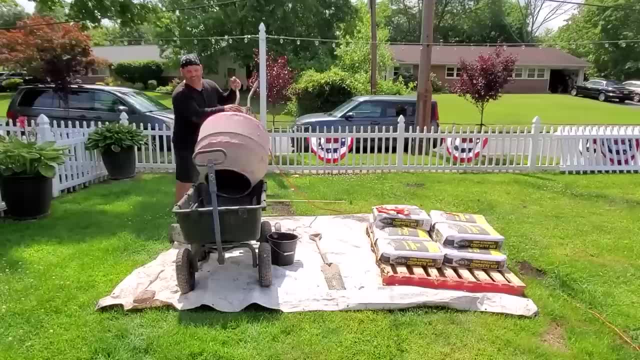 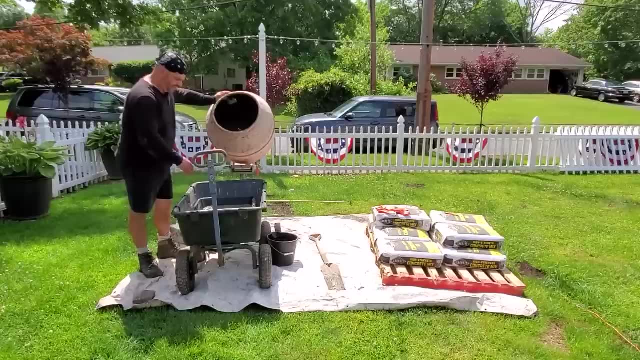 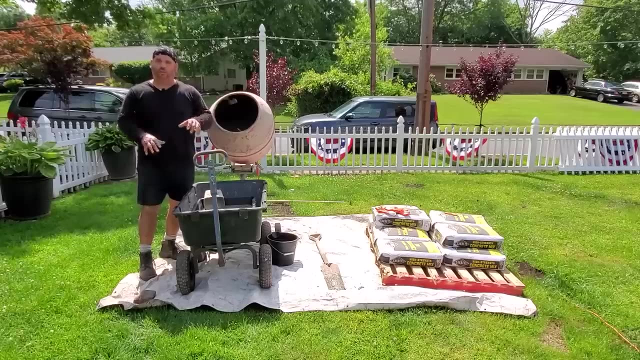 okay, and I think that does it. yep, got all stood up and I think it's a pretty good consistency. I lost Jackie. she's the expert on this, so what I'm gonna do is I'm gonna wheel this over and she's gonna show you how to work it into the form. 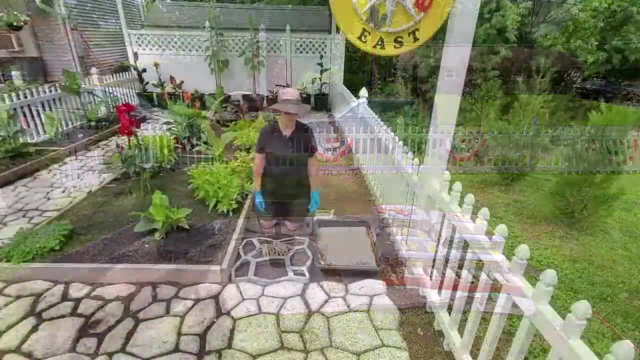 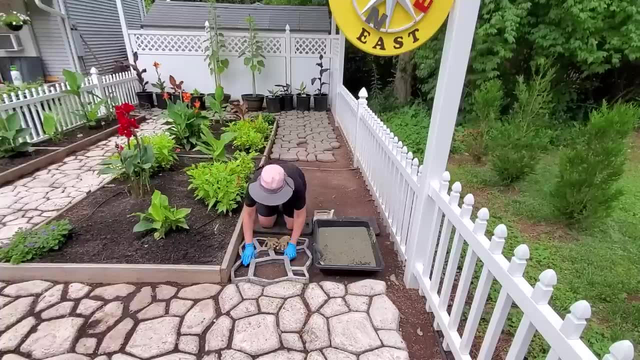 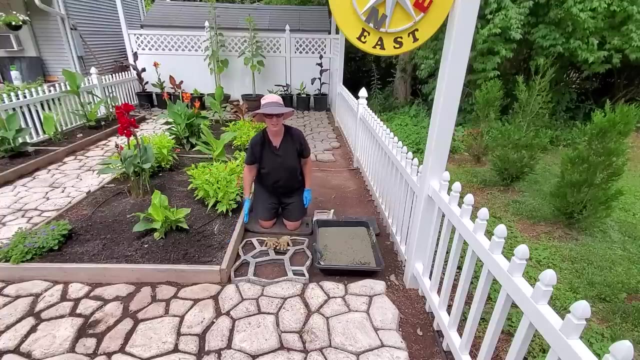 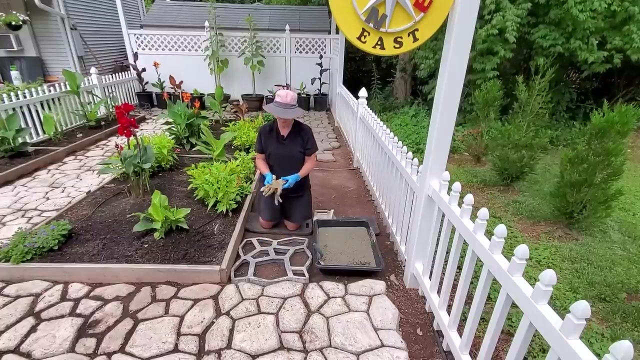 okay. so Dan got us our concrete mix and I have the form and we're gonna press it up against the stones that we did before, so it matches nicely. it's against a piece of wood, which makes it straight, and what I like to do is, as Dan mentioned about the chemical burns, what I like to do to 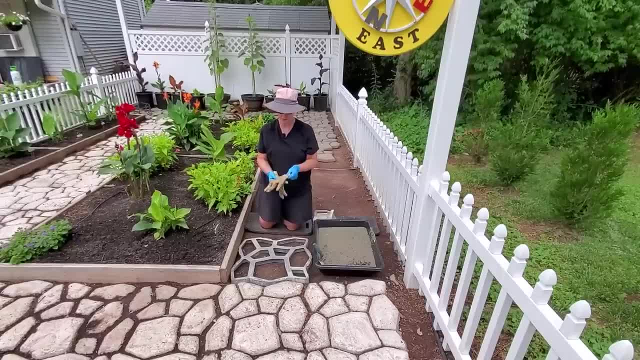 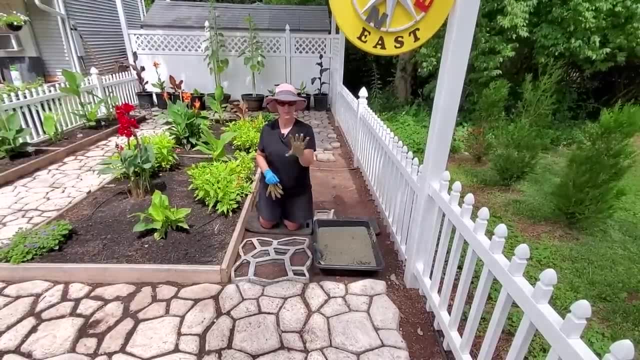 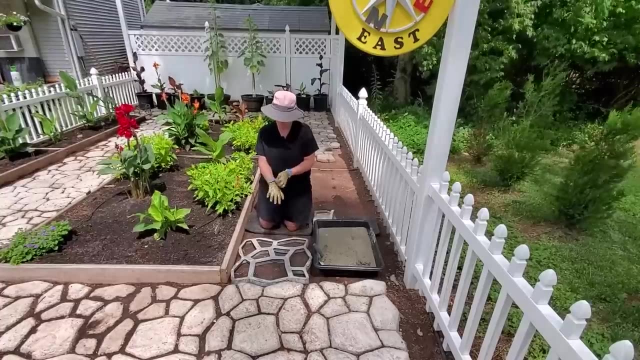 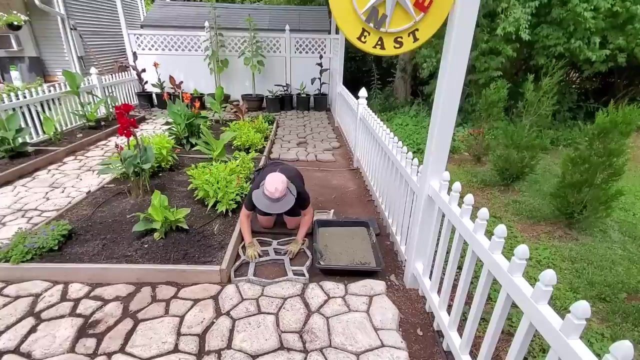 protect myself is. I wear latex gloves underneath my rubber work gloves and you can see I'm using a master. it's a little hot, especially on a hot day, but you know what it's worth- the protection. okay, all right, so make sure it's pressed up against both sides, make it straight and make it so it ends where you left off. okay, now I have a trowel really only when I have them in the middle of the floor, so I have to to get my hands on it normally. and then, and then you want to move them up, come up on the ground, and then you want to move them up on the ground and just press it in, and then you want to move them up, and then you want to move them up, hold it in and then really crush them and writing that you don't need to do it. 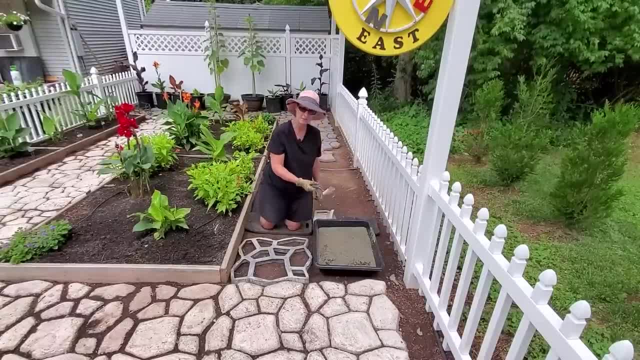 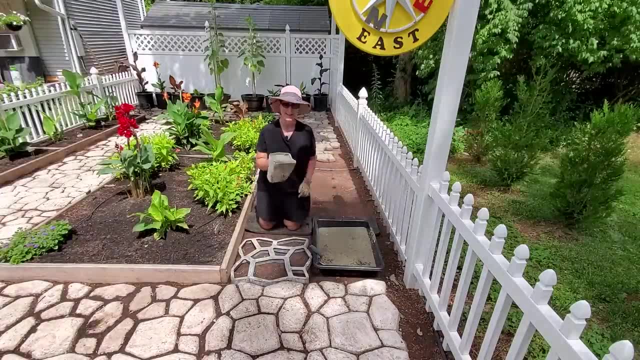 off. okay, now i have a trowel. really, all you need is a trowel. but what i like to do when i have big sections like this is i use my handy dandy scoop. i always have a handy dandy scoop, and this is what. 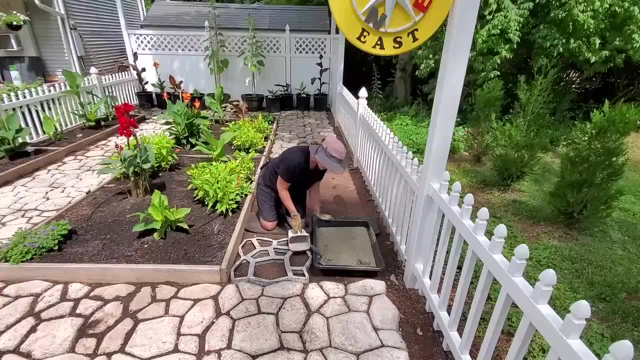 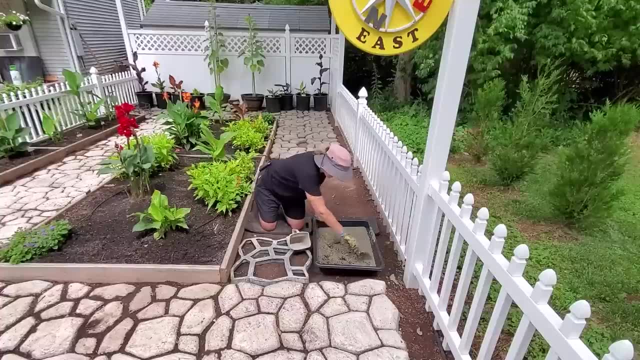 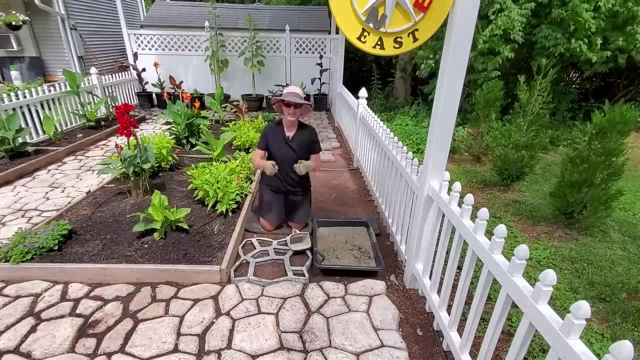 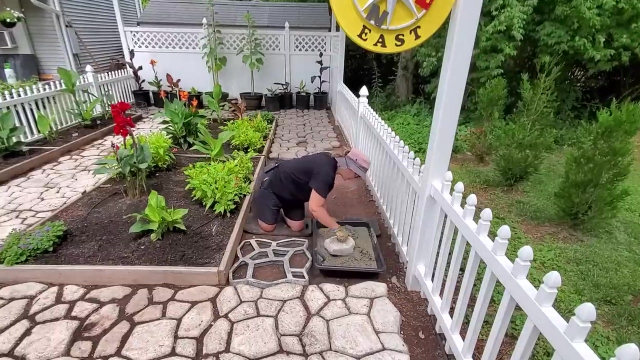 i use for concrete work. so the consistency first of all. check the consistency and make sure it's right. this actually looks perfect. it's not too dry and it's not too wet, and this baby bear says it's perfect. so you scoop up a large amount and i'm going to go for the biggest stone here. 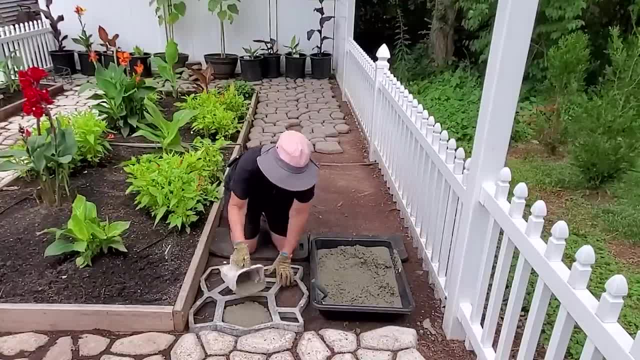 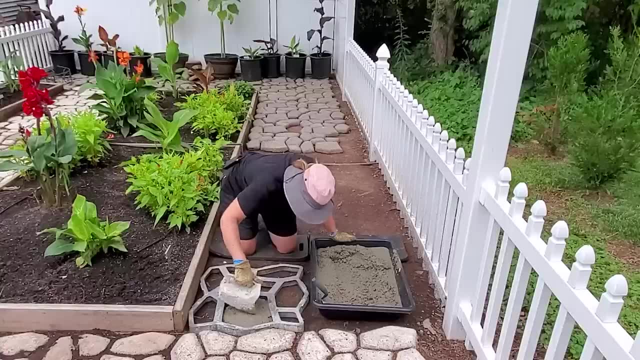 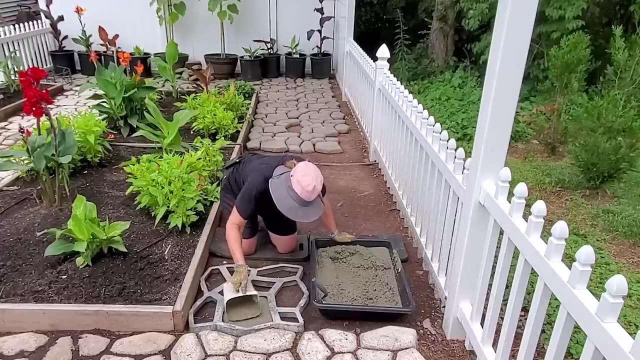 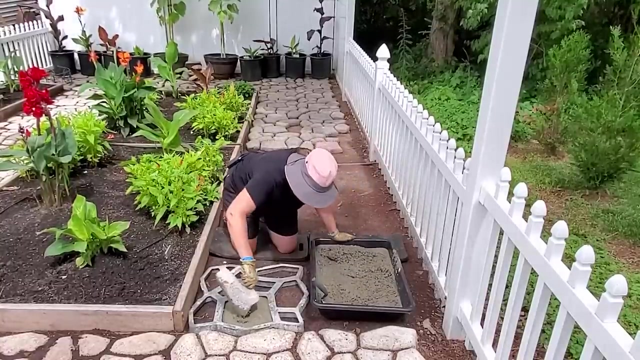 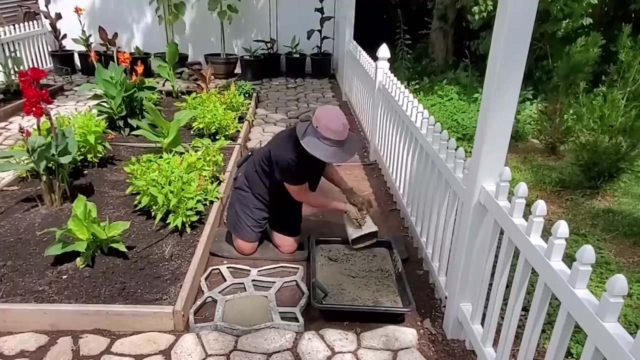 kind of pack it in a little bit with the scoop. you'll use the trowel to get into the corners. see, it's a little bit, there's a little bit of slurry there. just scoop a little bit more and then make it nice and level. now when you get that little bit that needs in that corner. 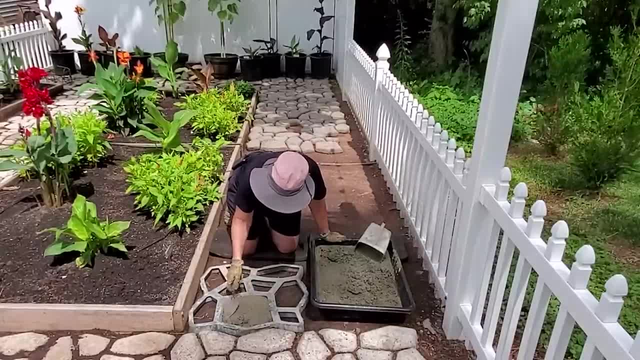 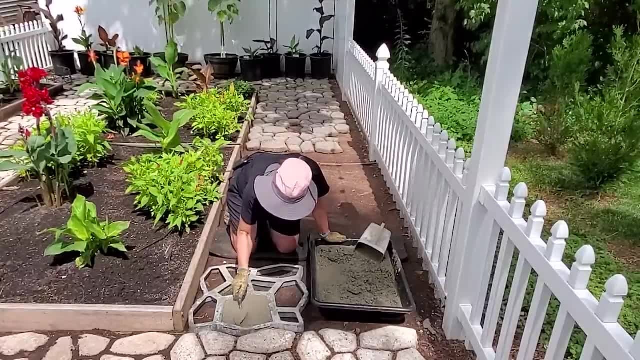 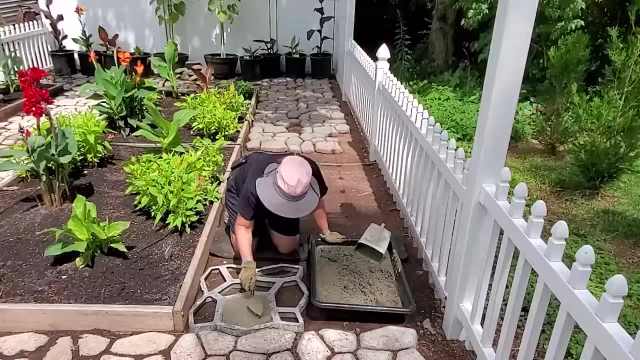 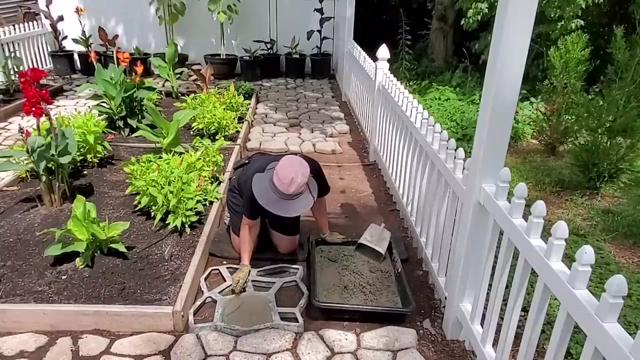 you take the trowel and you kind of just pack it in there and you pat it down as you go, put a little bit more in that corner and just kind of focus on the corners. that's the key thing at first. you can always pack more on top and it is going to level out according to the ground. 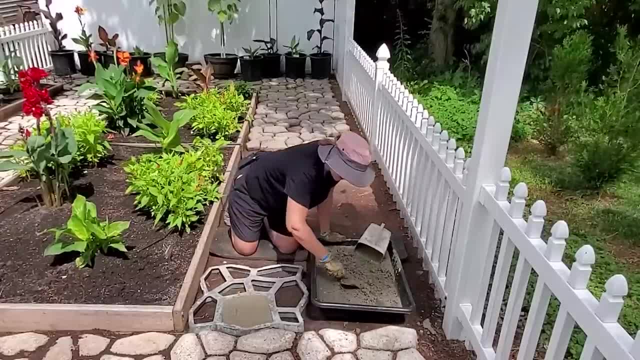 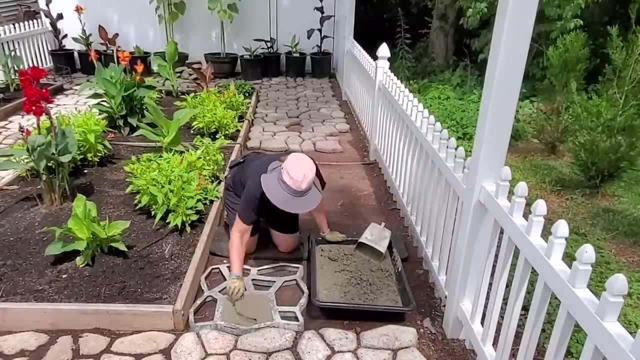 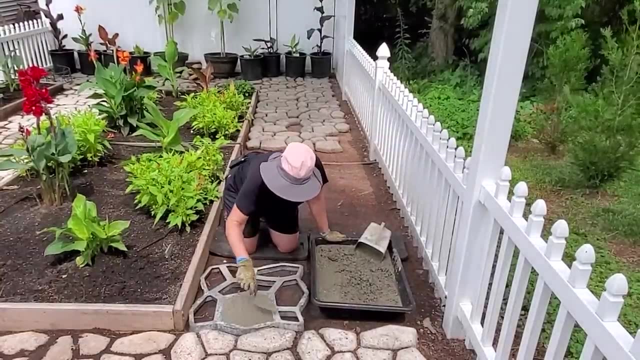 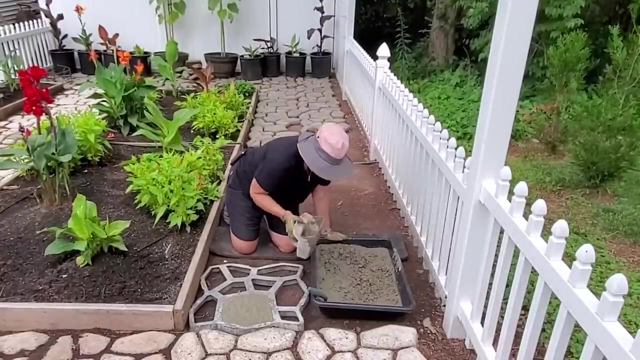 that's what's the beauty of this template. i need a little bit more and take a little bit more there and you can always go back. so if say, right now, i'm okay with that. i'm actually going to put a little bit more on there, but i'm going to continue to show you the different stones. so we're going to do this stone. 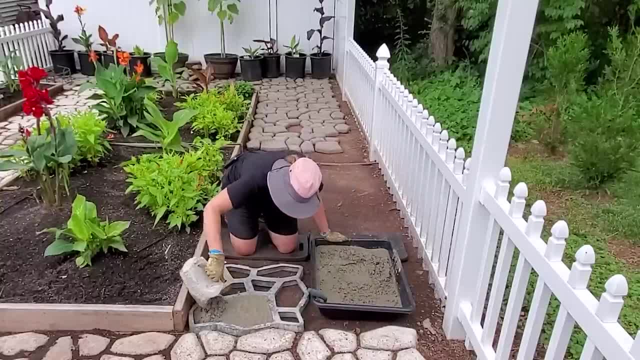 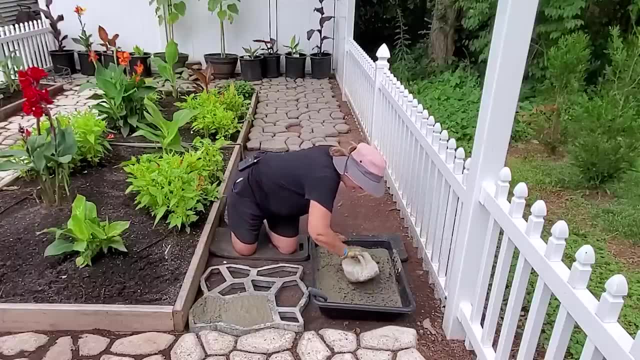 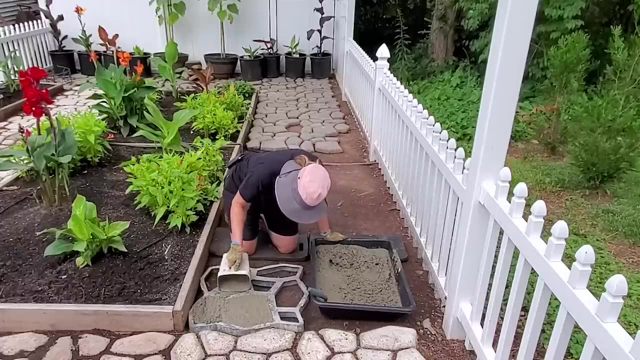 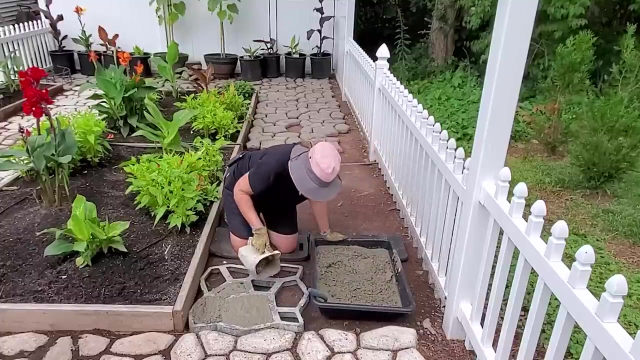 and you can continue doing it, so you don't keep it as neat, but you'll get a lot more done quicker. right now that's kind of neat and you don't have to do that. see like that, just pack it in as best possible. we're going to see how much we can fit in here. 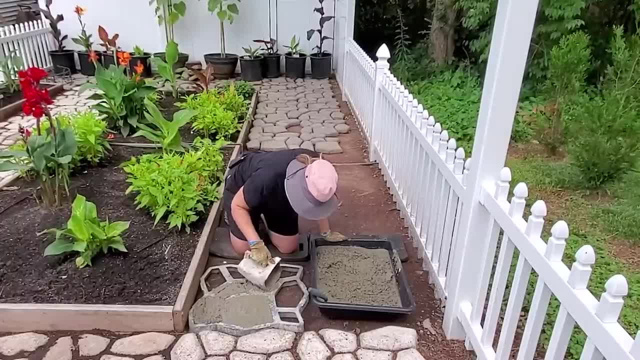 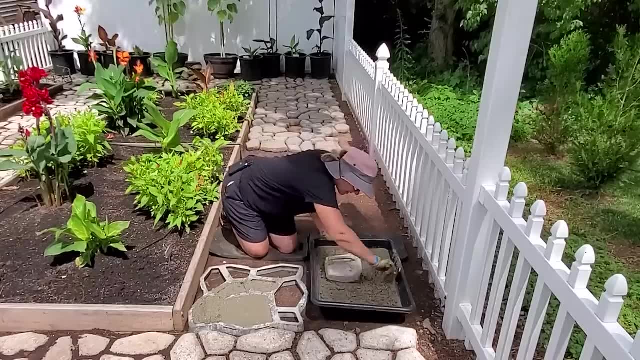 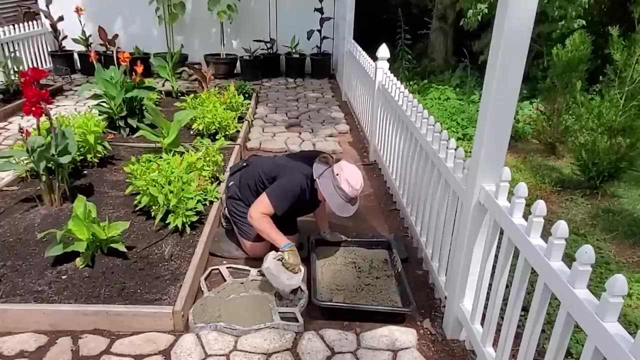 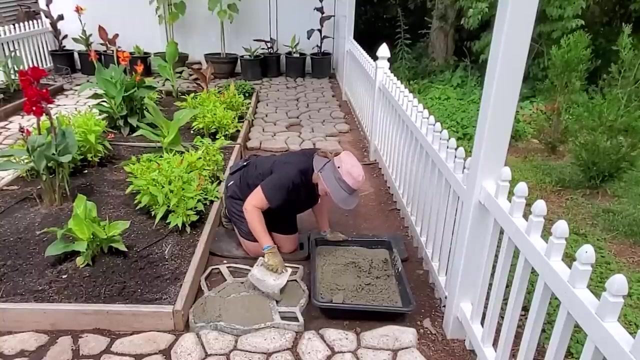 i think we're going to get a little bit more than that 80 pound bag for one template, but we're going to see- don't chance on it. if you need it, take it. there's another pretty big stone. just keep packing it in. like i said, the corners are very, very important. 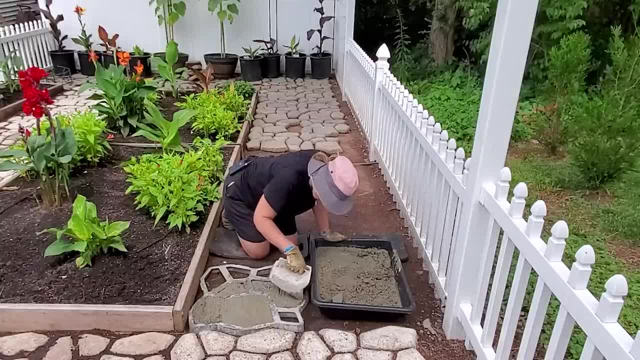 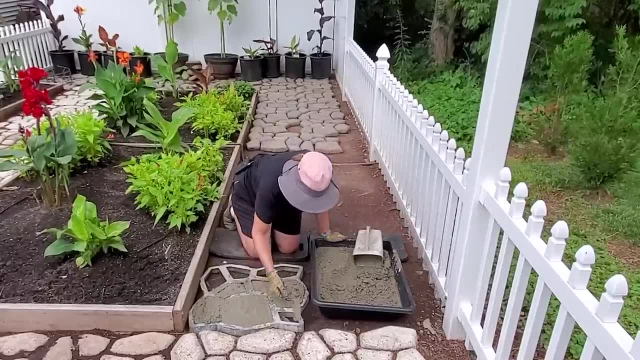 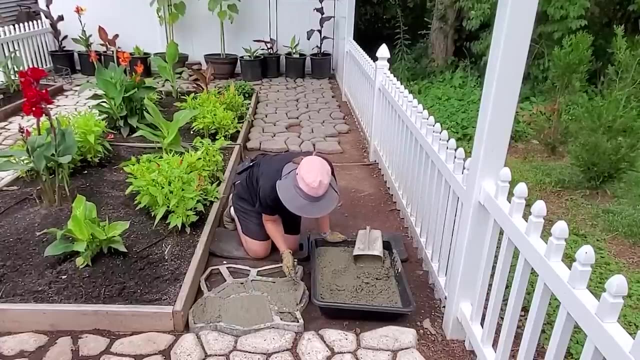 and if you put too much in like this may have a little bit too much. what you do is you take the trowel and you scoop it up and you put it in the next one. now there may be dig marks in here, but, like i said, what you do. 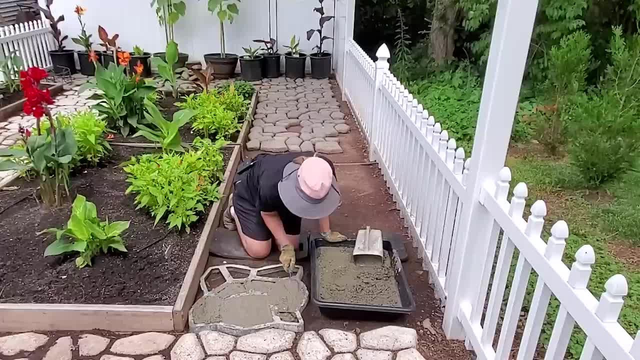 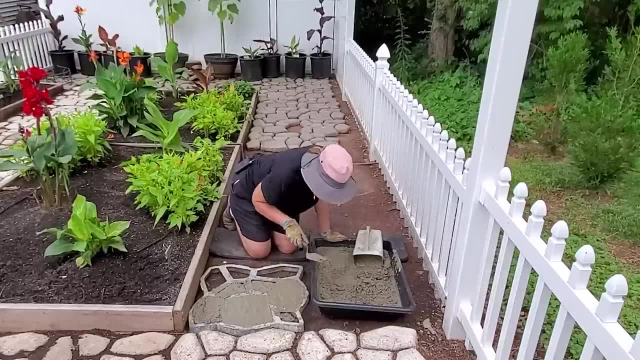 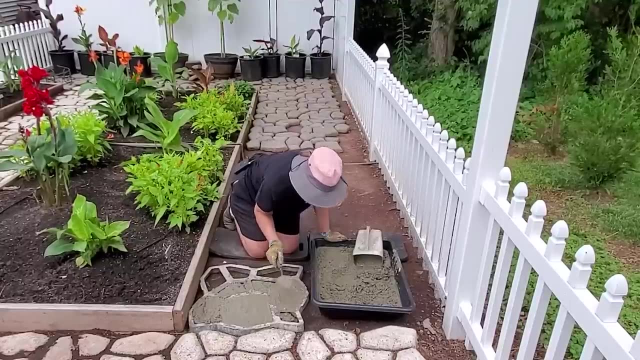 is you just keep packing it down and it flattens it out. and if you need just a little bit in the corner, take your trowel, pack it down, and i think that stone is good. if it's going to be a little stone like this, take your trowel. i think the scoop 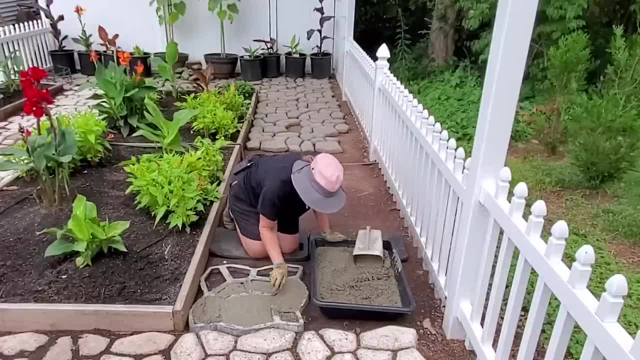 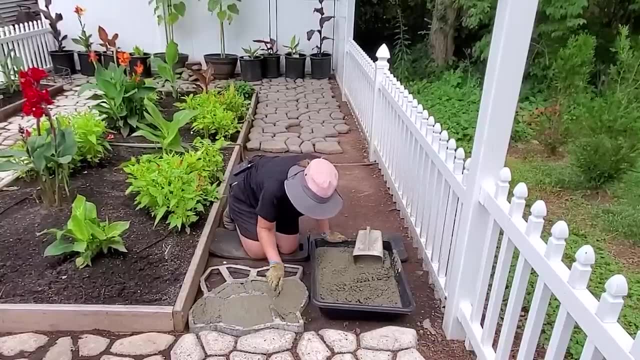 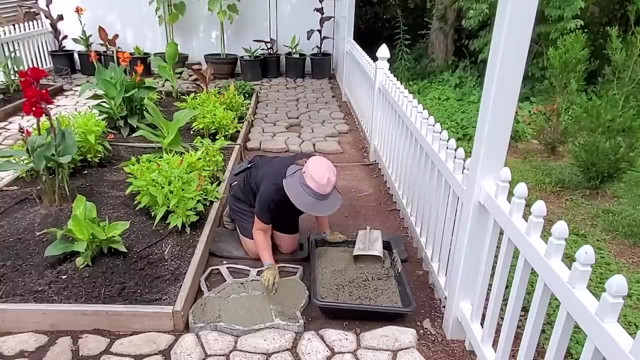 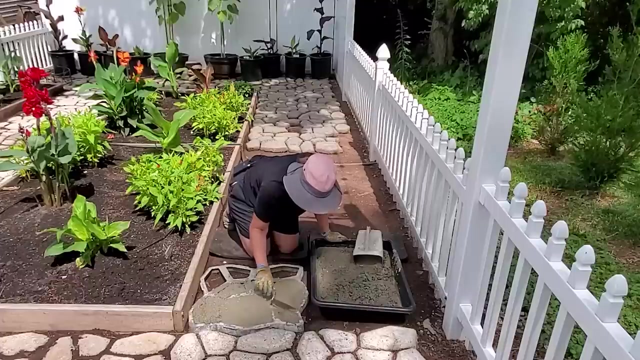 is going to be a little bit too big for that. just keep packing it. it's really all about packing it down. i think that might be too much. there we go, so let's see what i have here. okay, for now. i think that's good. i think i'm going to come back to that a. 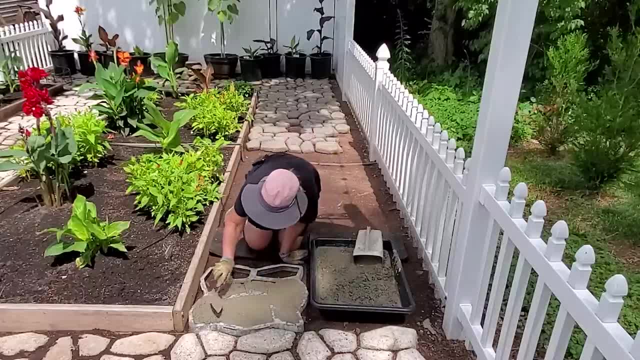 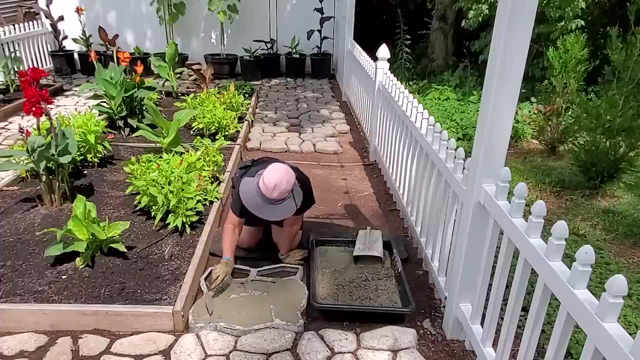 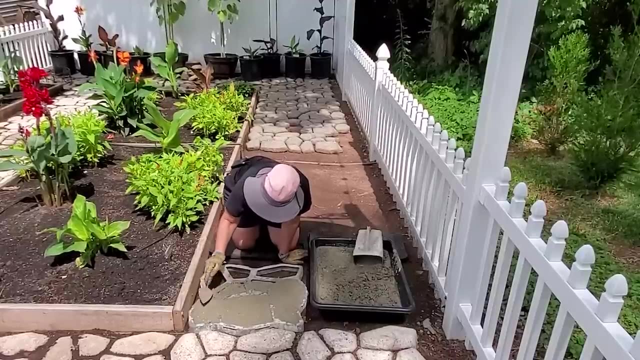 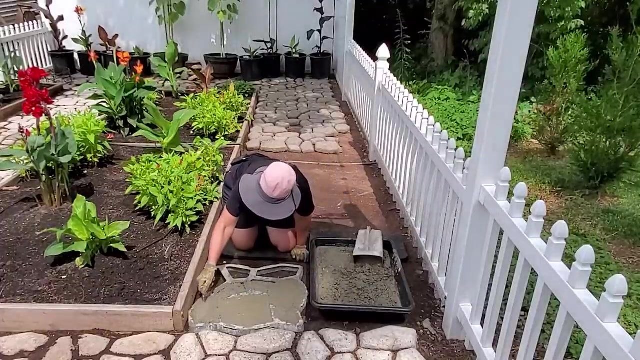 little bit later, when i'm done with everything else, let's pack this down, get that in the corner, pack it with the with the trowel. that's the beauty of having this trowel with the pointed edge. okay, a little bit more in there And after a while you'll get the hang of it as to how much you're going to need per. 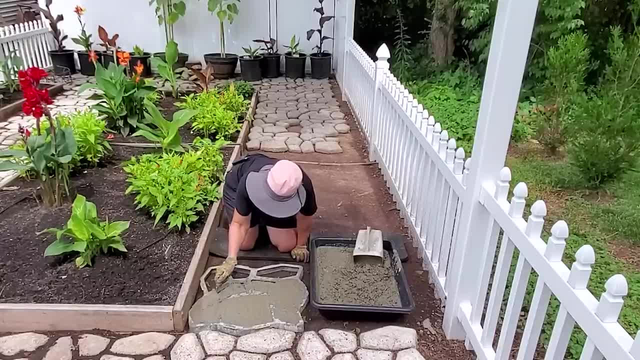 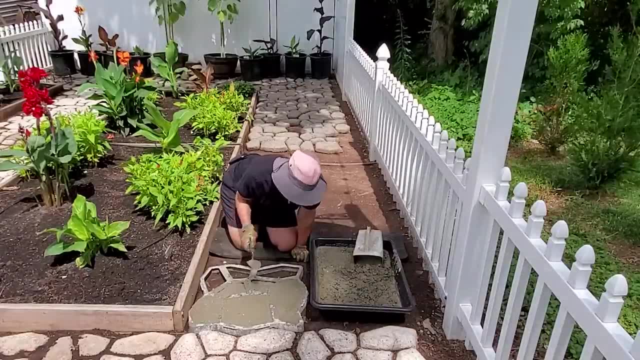 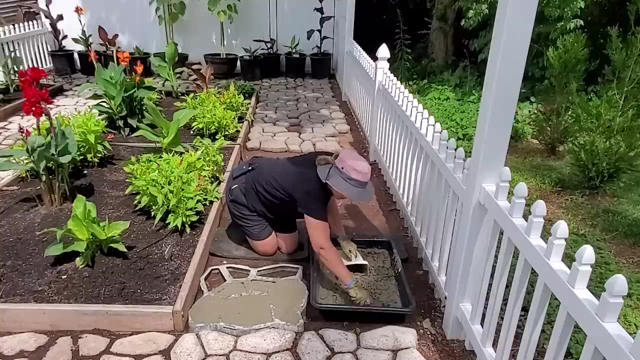 stone. See, there's a little bit too much in there, so I'm going to pack it down just to make sure. And I'm going to pack this down And you kind of have to work a little quick with this, because the cement will dry and 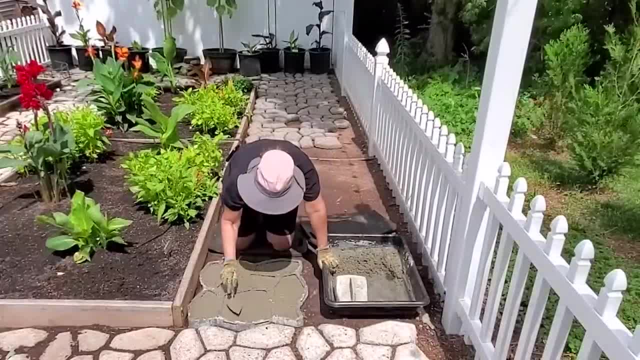 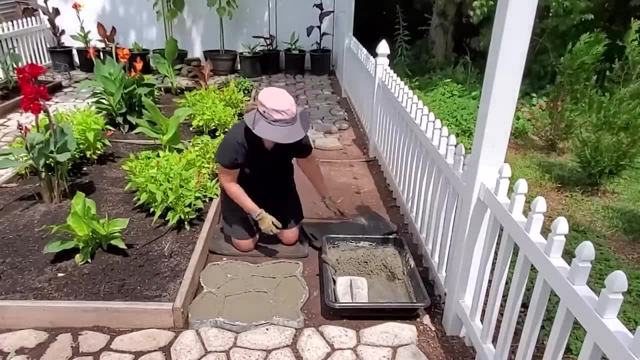 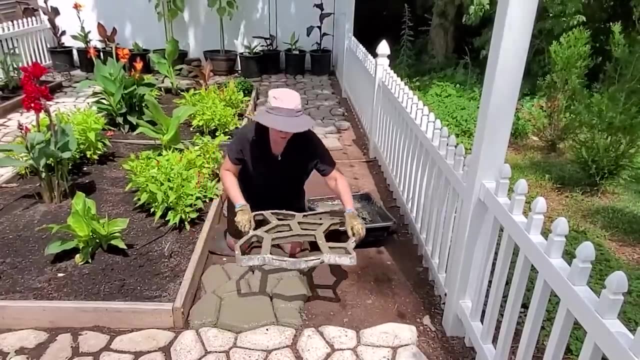 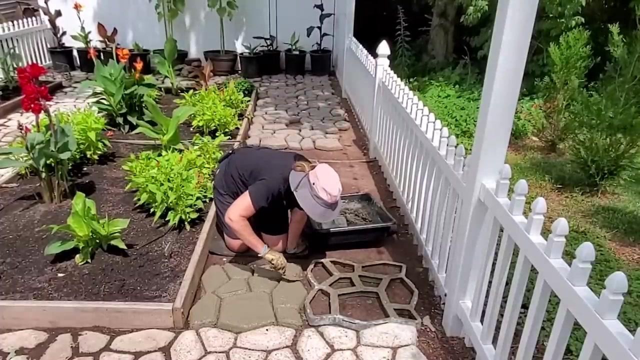 you certainly don't want that to happen. Okay, so I think we're ready. So we're going to actually move this bucket, take the form off, place it next to it, take the trowel and start patting down the sides to make sure that all the lines are. 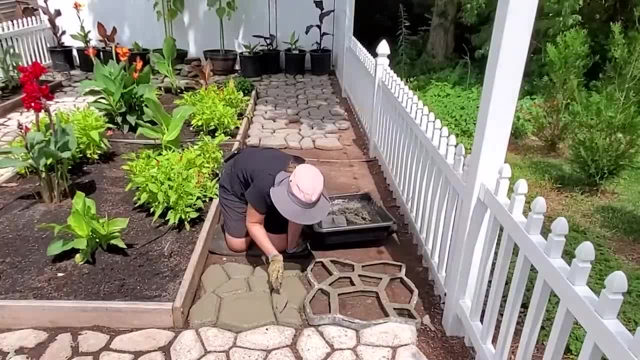 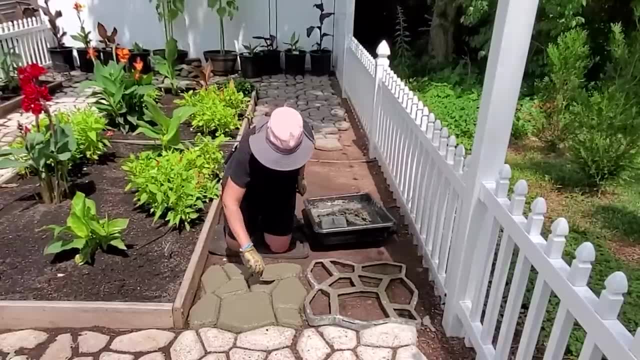 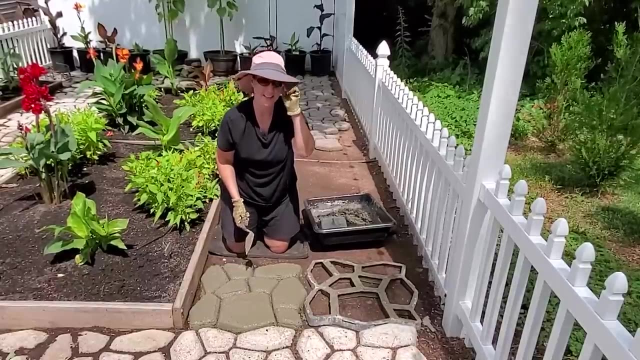 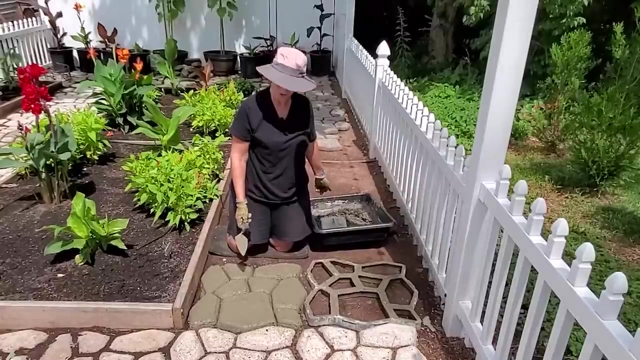 removed. Okay, Now, there's not going to be a lot of lines, but if there are any lines, you don't want them to show that it was an actual template. You want them to think that it's actually stones. All right, so I see that I actually have a little bit more than just this one template. 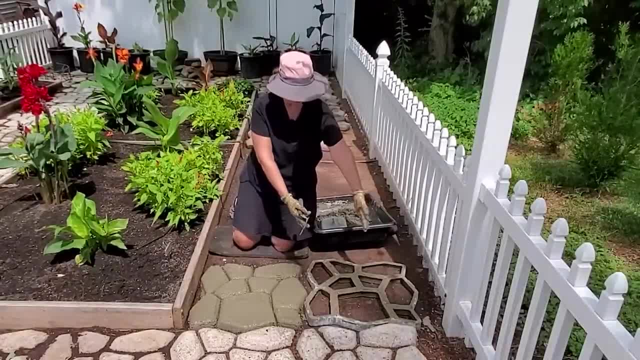 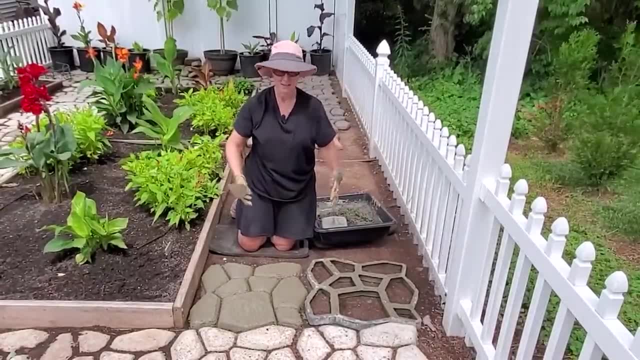 that I can use this for. So what I'm going to do is just place this down, Okay, So what I'm going to do is just place this next to it. You could do a half turn if you want, but we like to have a consistent path. the design: 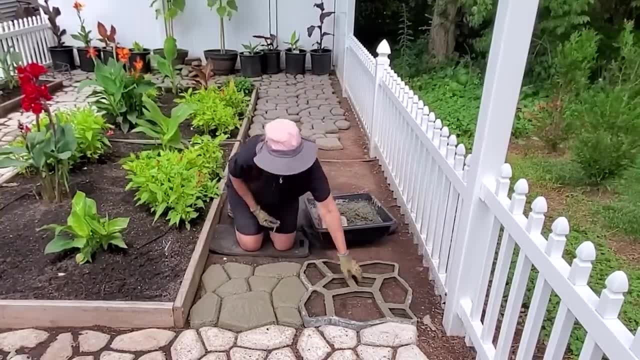 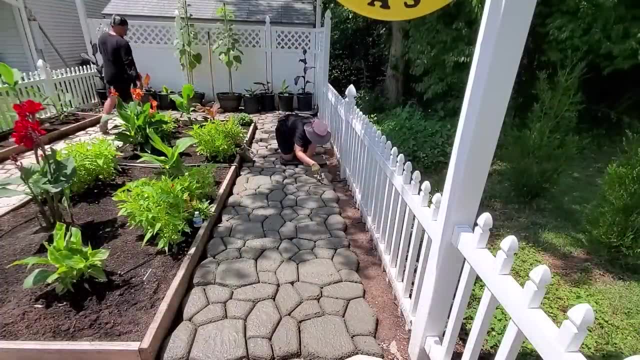 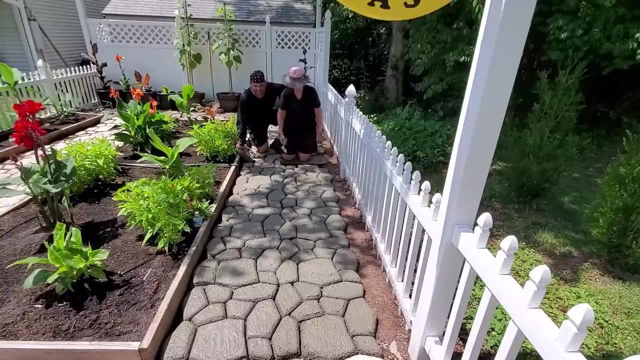 So we just place it right next to it and then I'm going to continue. Hey man, it's coming out great. Yeah, it is coming out pretty good. Yeah, Only 22 more to go. All right, All right. 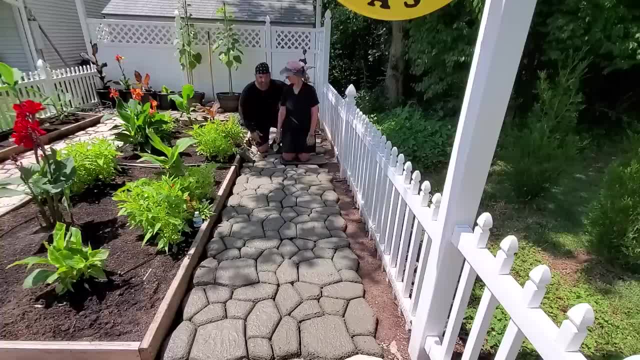 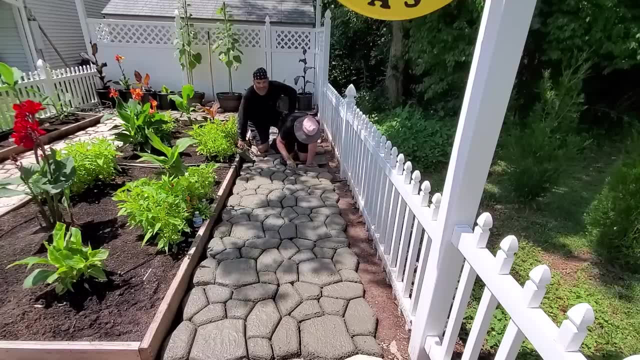 All right, That's about it. Okay, All right. All right, You want to take a stab at this? Oh, absolutely, You want to mix those 80-pound bags of concrete? No, I think I'll stick with this. 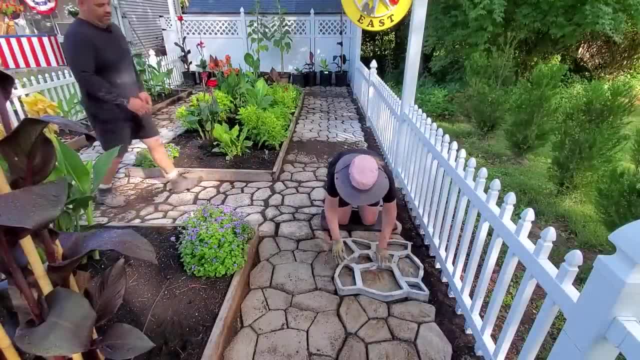 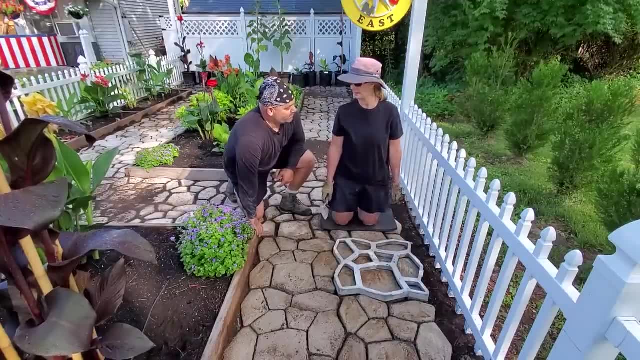 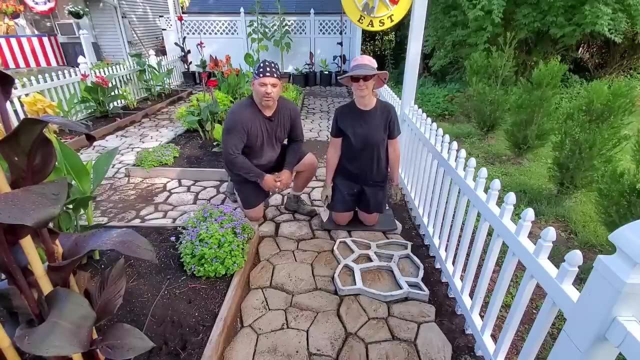 Last one. huh, Yeah, It's been a long day, right, Ben, I know, but you know what It's worth it: It looks great. Yeah, it does, Yeah, do. now is we got to let the concrete cure. so we're going to keep spraying it down or misting. 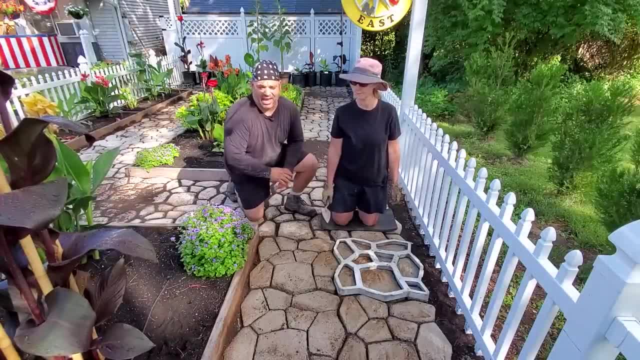 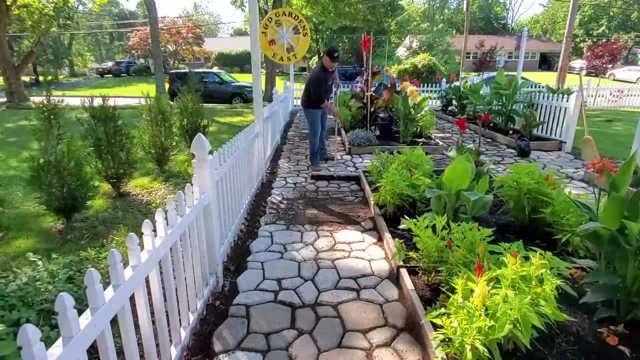 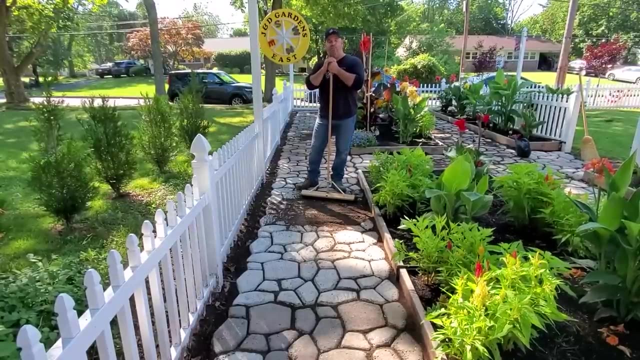 it with some water, so it cures slowly for the next few days and we'll be back later and show you how to finish up. okay, so it's been about three days and the concrete is curing nicely and it's safe to walk on, and all we have to do now is literally fill in the gaps. 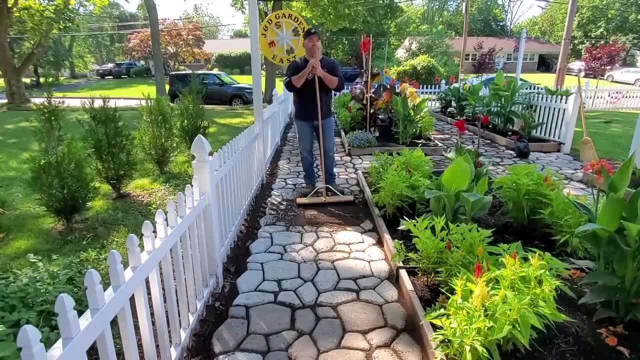 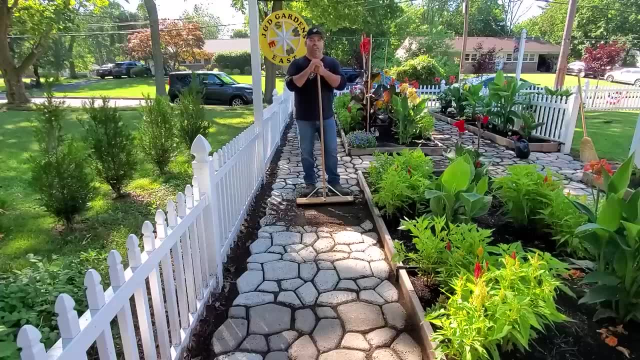 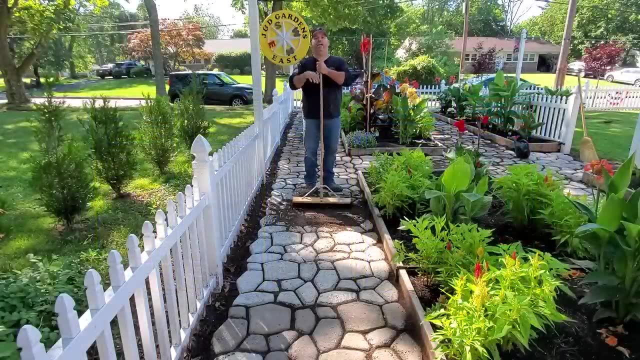 but i want to talk to you a quick thing about color. now, if you're thinking about adding color to your pathway companies, like quick read, make a dire solution that come in a variety of different colors. now, this solution is added while you're mixing the concrete, but it's something that you 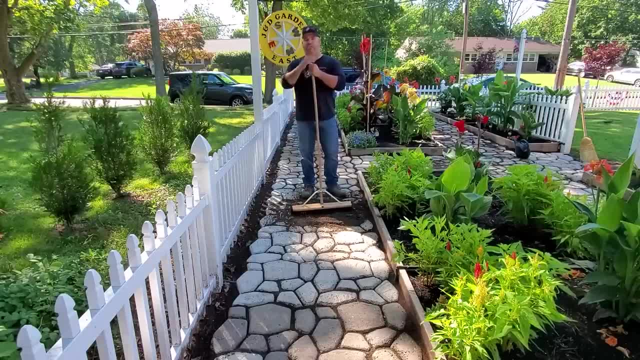 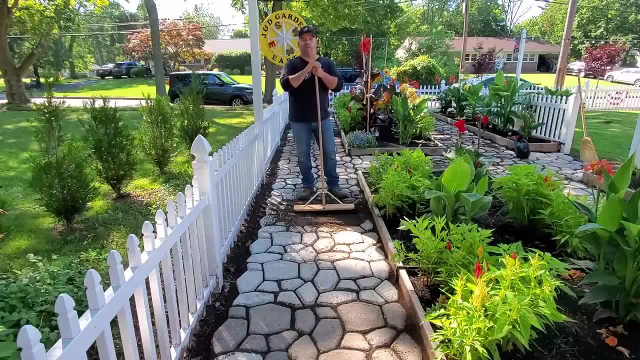 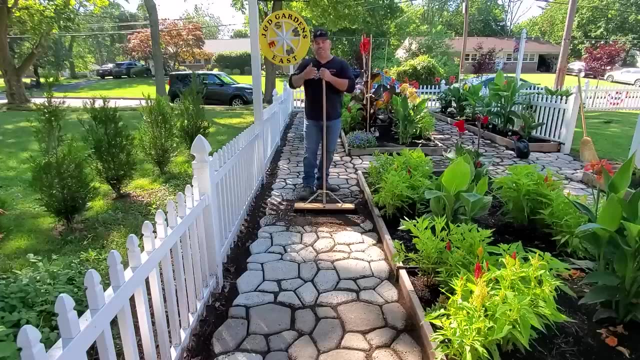 might want to take into consideration very early on when budgeting for your pathway. each- uh each- bottle of the solution will run you about six dollars or so- i think that's the going rate- and each bottle will do about two bags of 80 pound concrete. so let's use this as an example. we did about 32 bags of concrete. so half of that is 16 times six, that's about 96. so you're about close to a hundred dollars. actually will be more than a hundred dollars after taxes, so you really want to factor that in early on. it's not like a last minute thing or it's gonna just come out. it's. 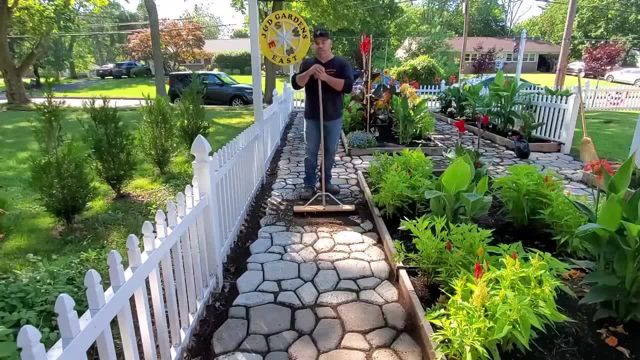 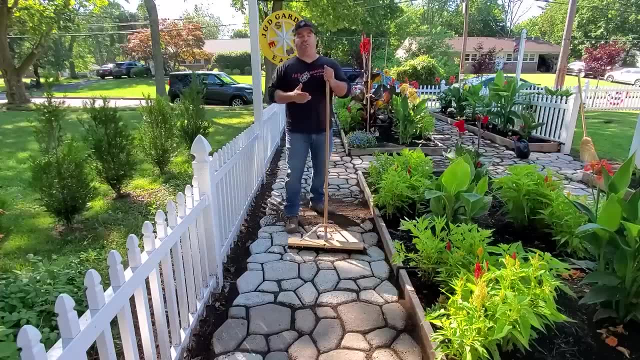 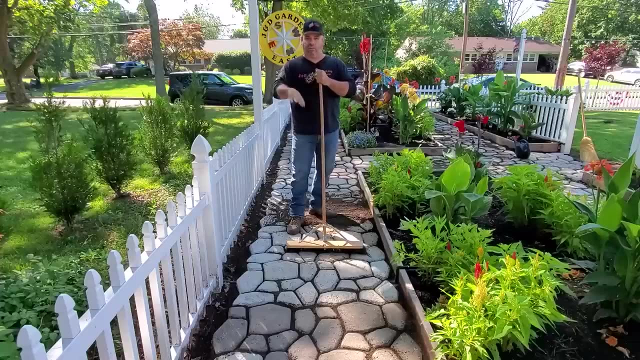 gonna hit you in the wild really bad now. we actually didn't use a uh any kind of tint and uh the reason why, as i said, we've been uh doing this uh pathway for years. we've actually done in different parts of our property, we've actually consolidated all here to uh, to garden east and, as you can see right here, the 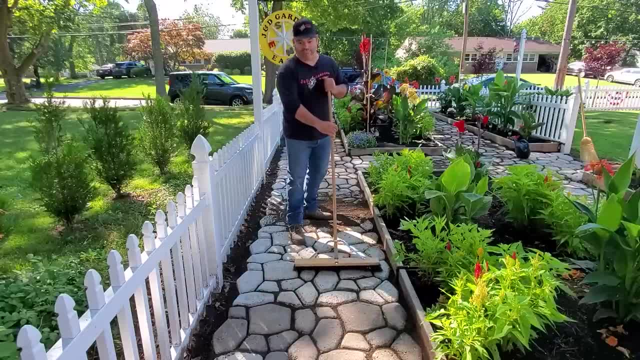 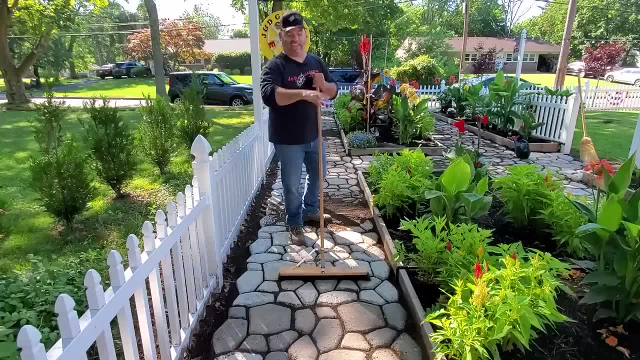 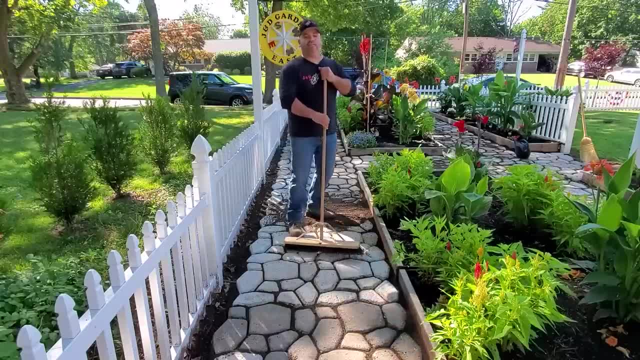 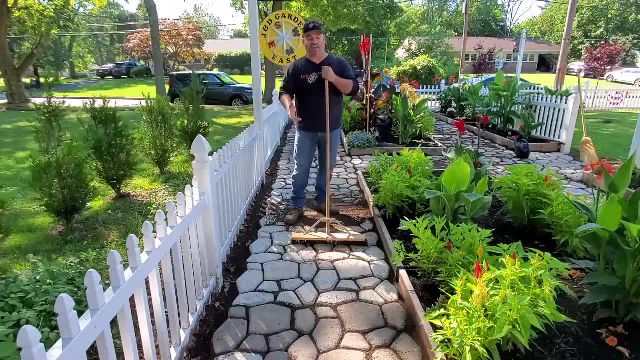 this is the newer concrete, so you see the white and the gray. now what we're going to be doing in the future is they actually make a concrete stain, which i've used, and it's something you spray on and it's a permanent and it works great, and we found that that would be a lot easier, so we're. 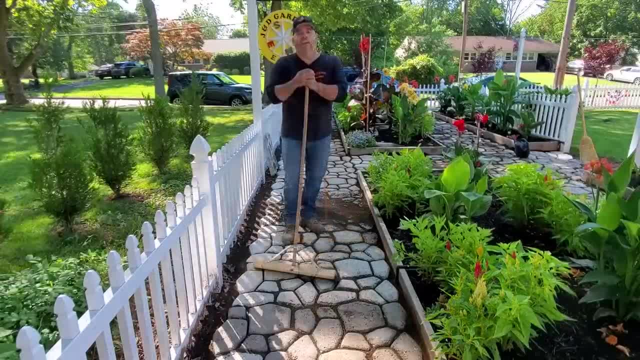 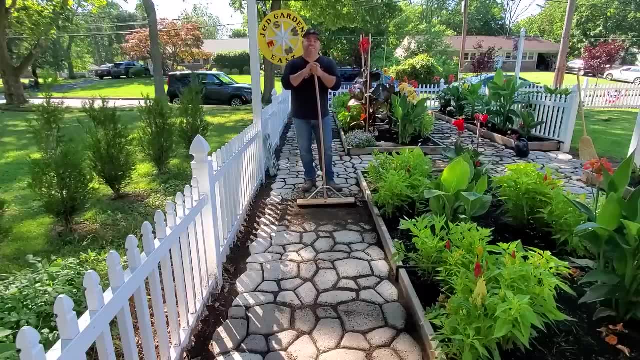 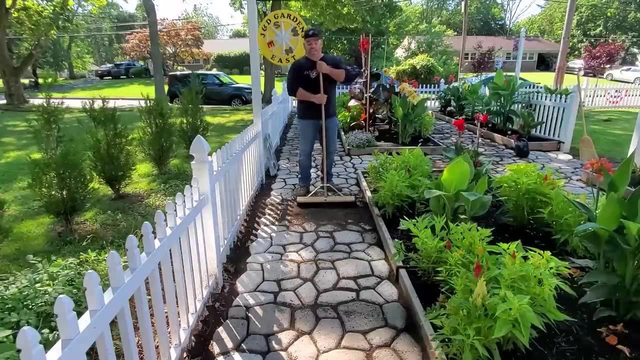 going to try to match the two together. so let's get back to filling in the gaps now. there's a couple of different ways of doing it. quicktree makes a product that's a polymeric jointing sand. say that three times real quick. it's actually called hardscape, and what it is? it's a. it's a. 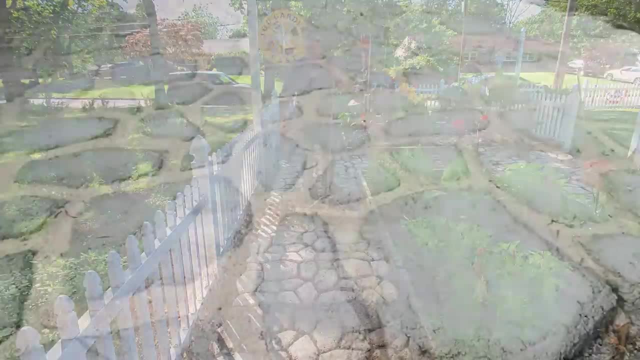 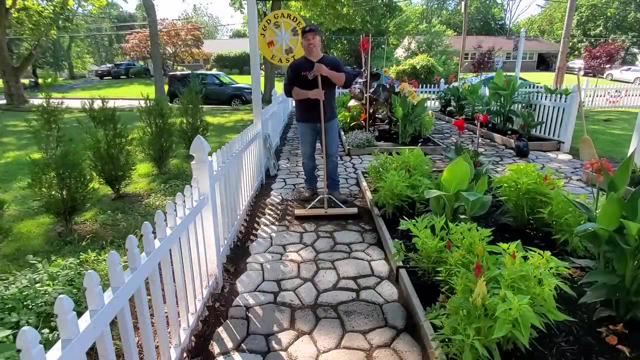 sand that you sweep in between the cracks or the gaps and you hose it down with water, and when it dries it'll act like a bonding agent and hold all the stones together, and a lot of people like that because they don't have to worry about the the stones moving at all. 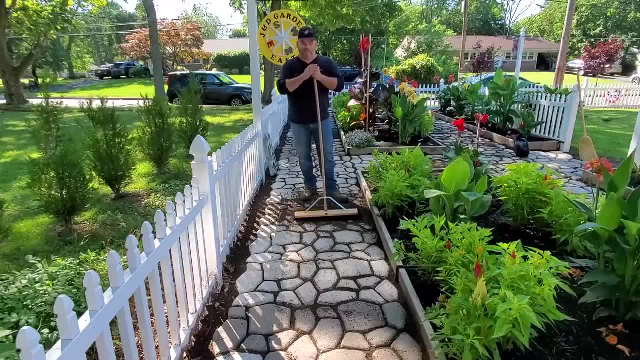 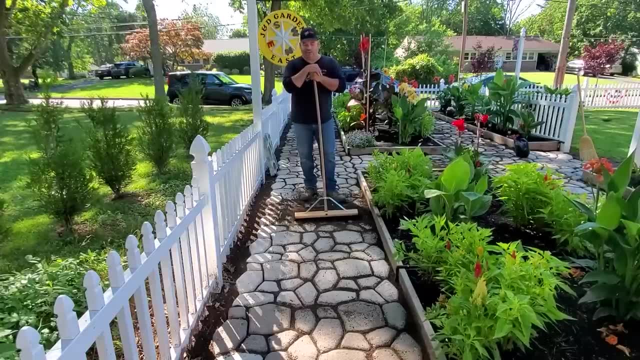 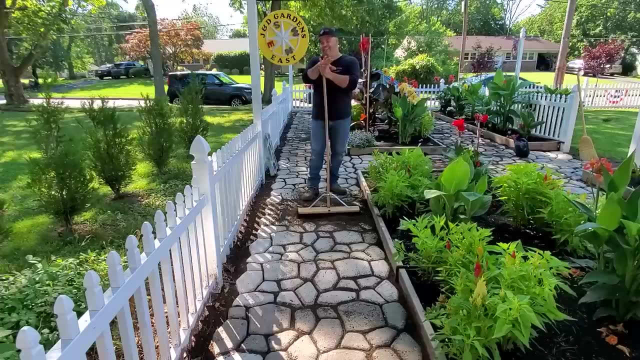 uh, but for us, uh, we actually don't like that too much because it uh it, there's too much gray in it. it kind of looks like concrete. it doesn't give that natural stone path. uh, that we want, uh, so we actually use, is regular top soil, and it's the same process. it just takes a. 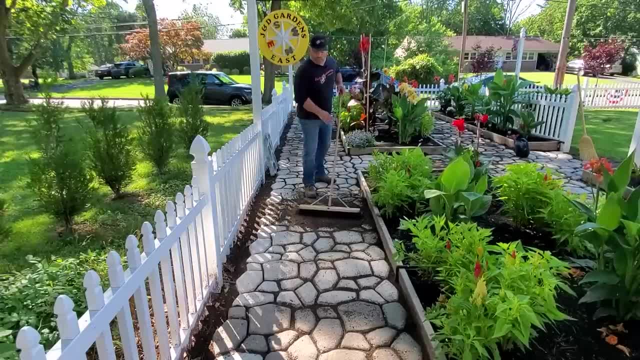 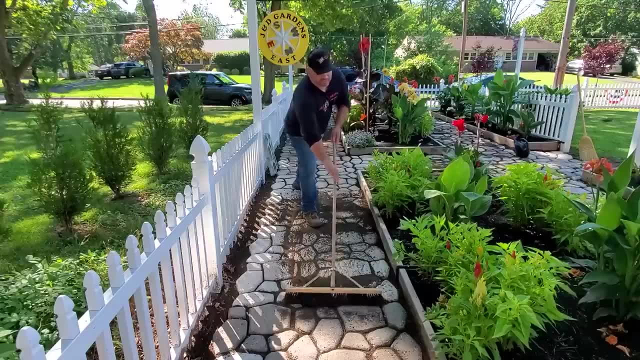 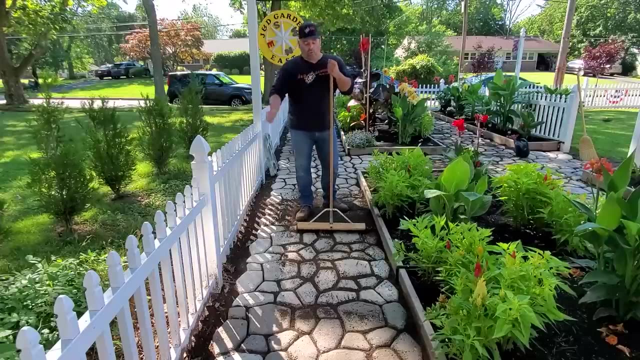 little longer. let me explain, since what you'll do is you'll want to sweep in between. if you can see I'm doing it, you'll sweep in between, and since it's just regular dirt, there's a lot of gaps underneath it. so what we'll do is we'll hose it down with water. 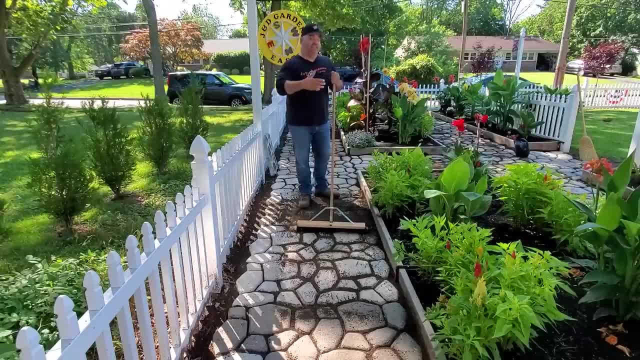 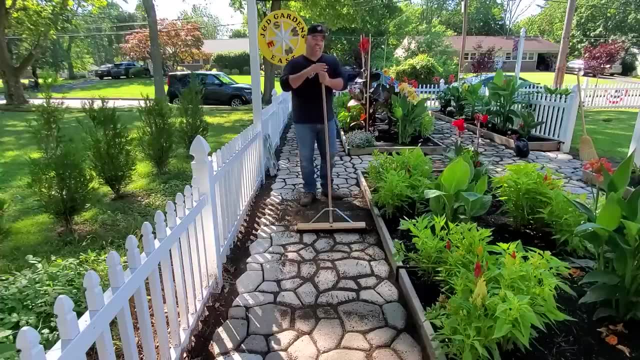 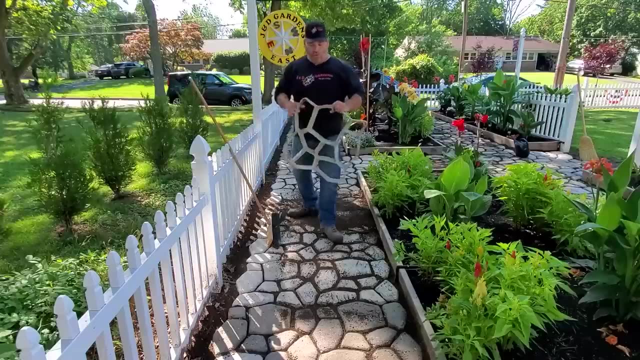 and then let it dry and then sweep in some more. eventually all the dirt will seep to the bottom and lock everything in place. so it does take a little while. something you can do to speed it up is that if you have your template, you'll want to pack down the sand or the dirt rather so you line. 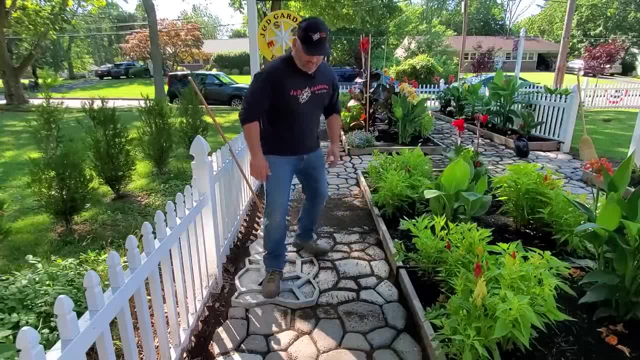 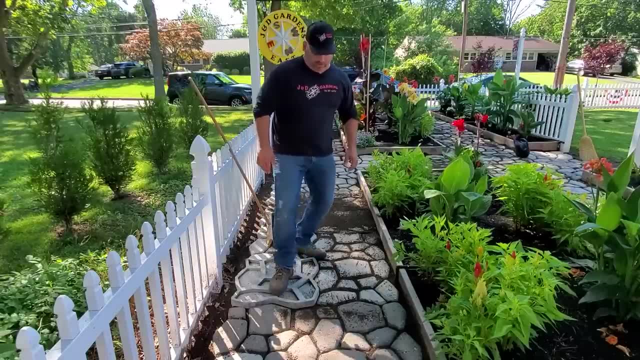 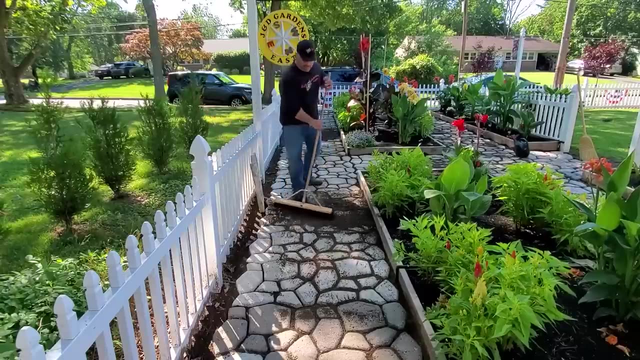 it up the way you want it, step on it and what it does. it actually will start packing down the sand for you and still add the water. it'll help lock it in, but, as you can see there, see it's packing it down. it takes a little while and then, like I said, you just keep adding more dirt. it'll fill in the top. 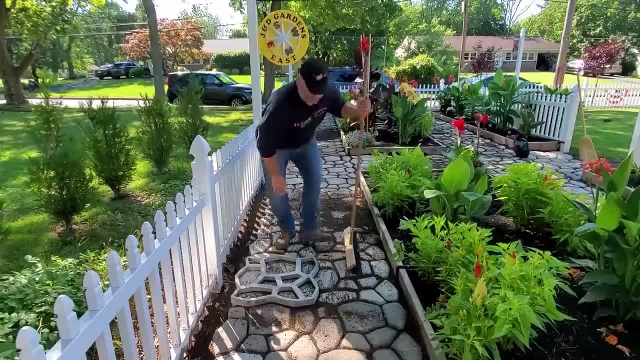 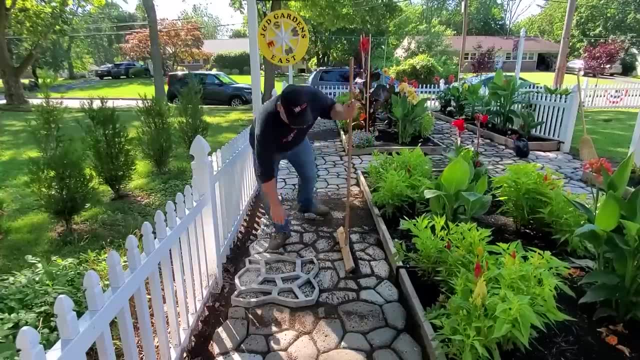 and again, when you see that you've packed it down, so it's getting there, nice. I've already done this down, so it's getting there, nice. I've already done this down, so it's getting there, nice. I've already done this, already done this a few times before we started filming, But you see how that looks. And then 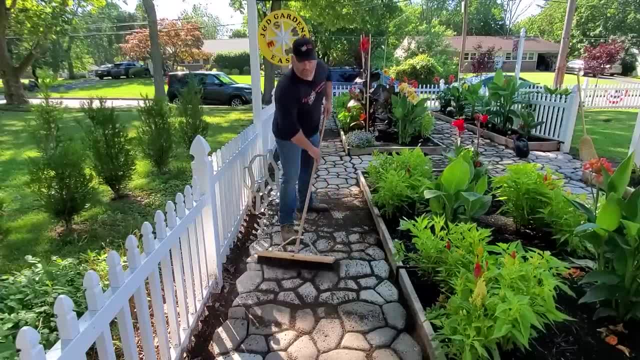 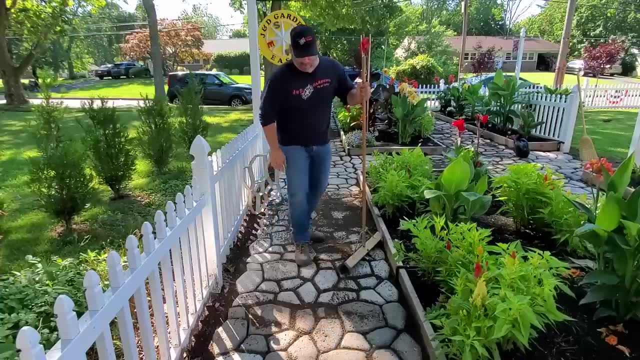 once you feel that you've gotten it. I'm not adding water right now because I don't want to make a muddy mess as we're filming, but you see, it'll actually help form the stones around, so you really get the kind of the country stone look that you're after. And, like I said, 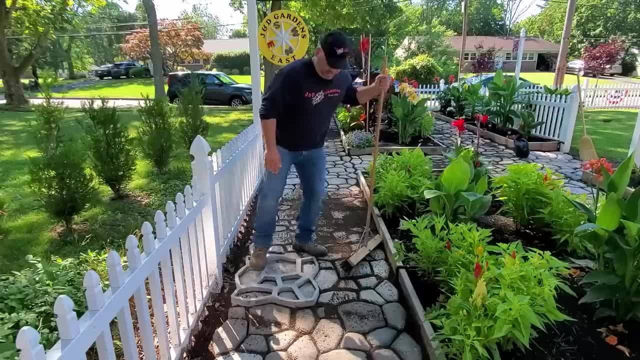 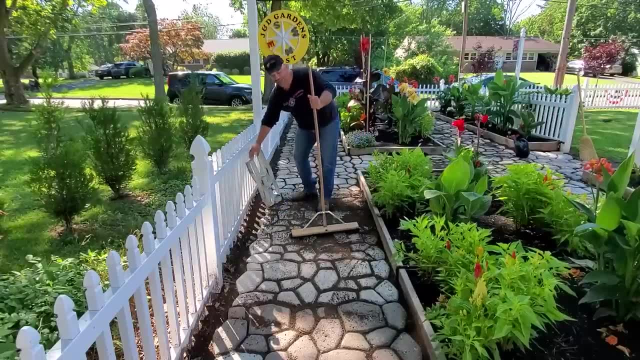 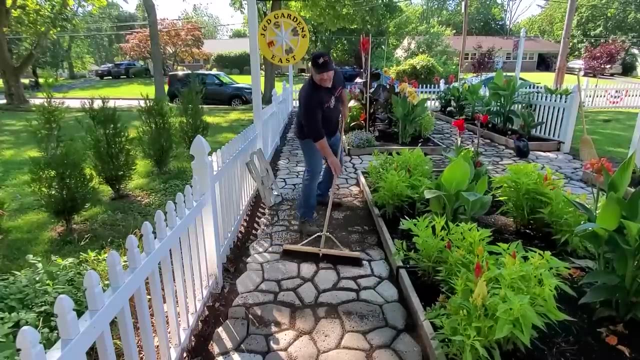 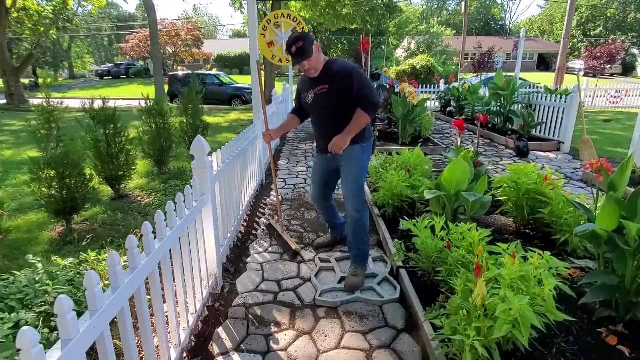 repeat it until you feel that everything's the look that you want. And don't try this while everything's wet. It'll just make a total mess. Just try one more so you get the look And you really see the stones are becoming pronounced. They look great, Form's tough. 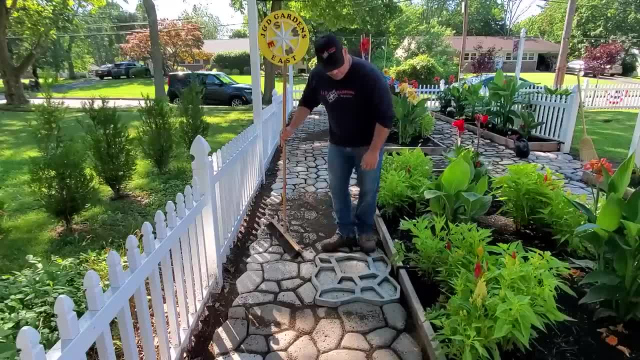 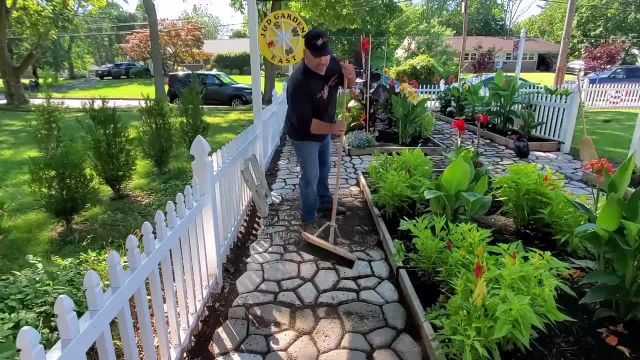 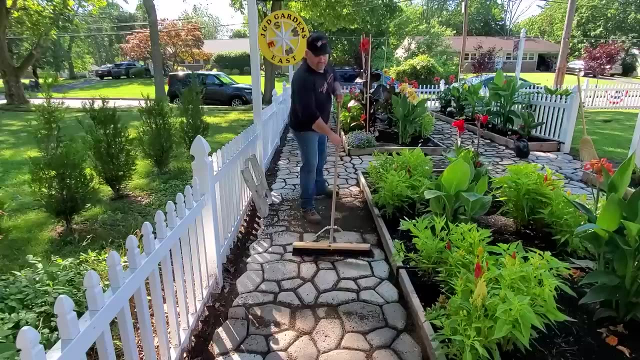 It can handle it. Just don't Don't get too crazy with it. Just really will define each stone And give you. there you go. Now I'm going to add some more water to it. I've already done some, but I'm going. 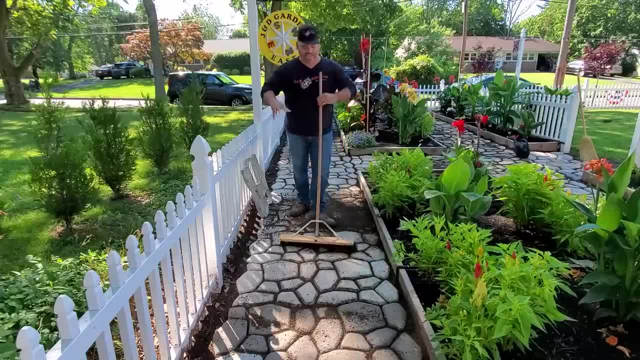 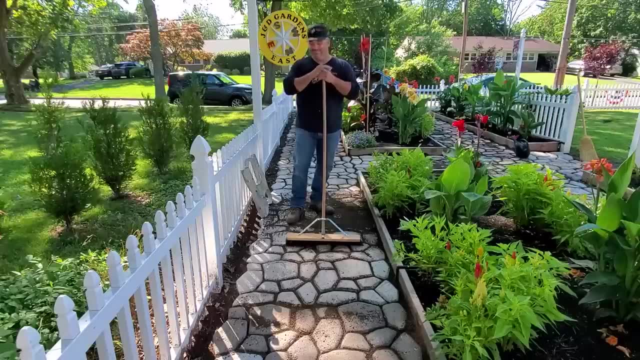 to add some more and do it a few more times, But it'll really get the stones nice and tight together And it'll work very similar to that polymer sand Now, Okay, Okay, So I just rip it out. So if you like the look of this, it doesn't come without its. 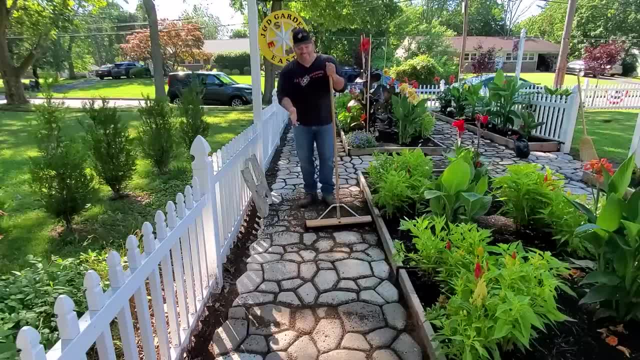 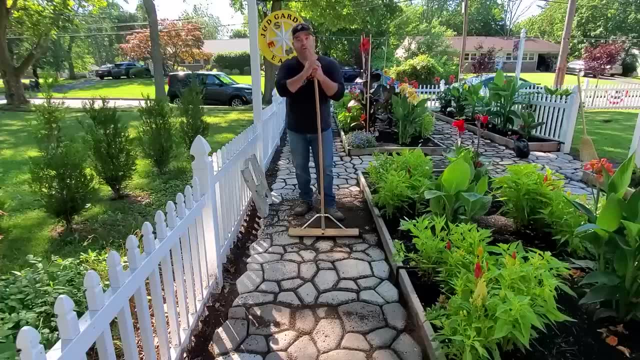 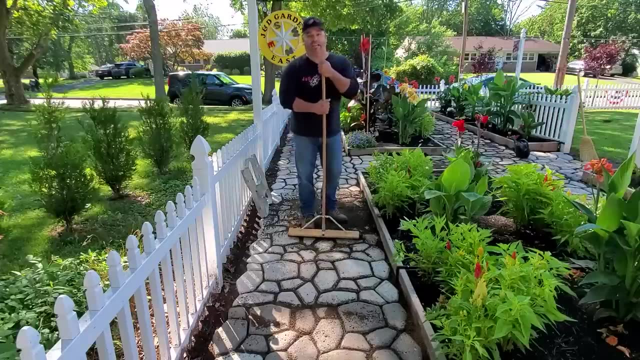 problems. And let me explain: This- is dirt in between. So what does that mean? It's very likely that you can get weeds, So it can be a little bit of an up keep coming through and taking out any weeds. So the best thing that we suggest to do, since we've been using 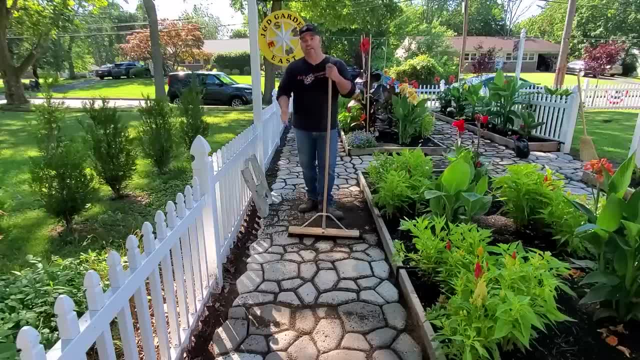 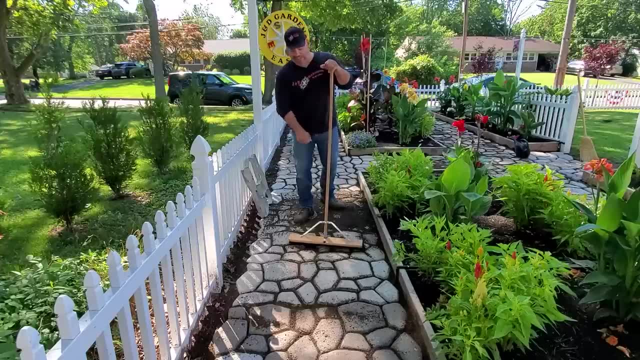 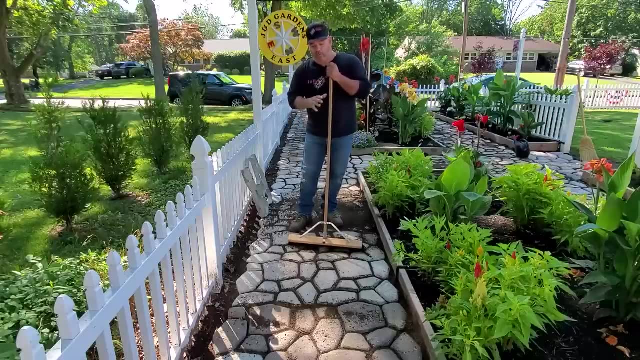 this forever is: every couple of weeks, come around with a watering can- make sure you've, and some kind of weed killer and just go through everything. just spray everything down. everything will go into the cracks, will kill off any kind of growth in there because you do not want to go away. 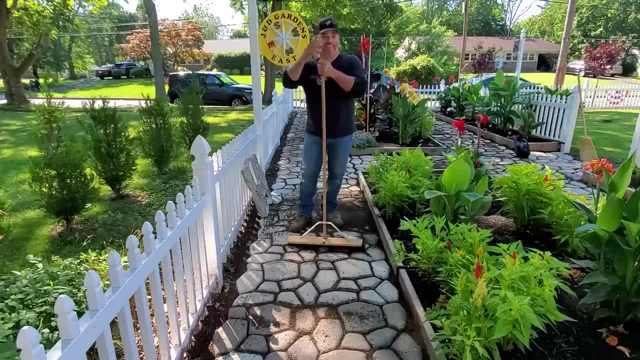 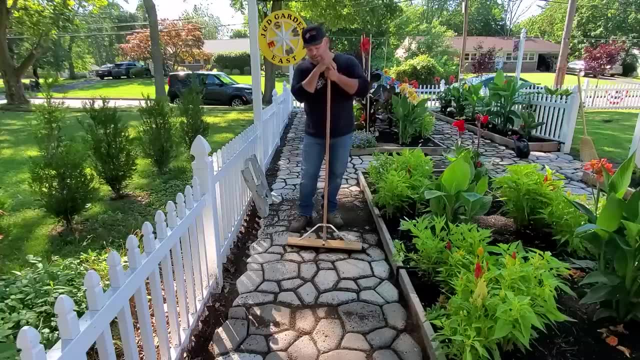 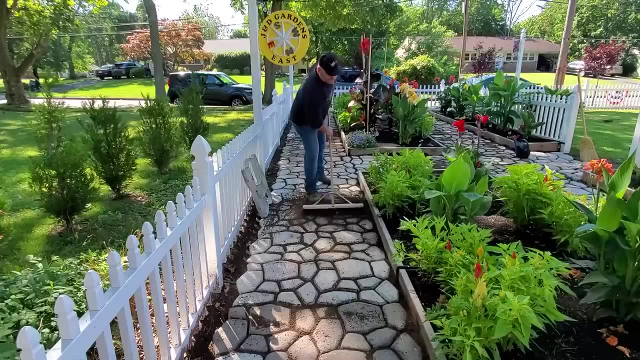 and forget about this and come back to a bunch of weeds, because everyone knows weeds grow like weeds and they are relentless. so it's a little bit of upkeep, but I think that the end of the day, once you get it all and you fill in the gap, I think that the look is really amazing and like.